So let me get going here. 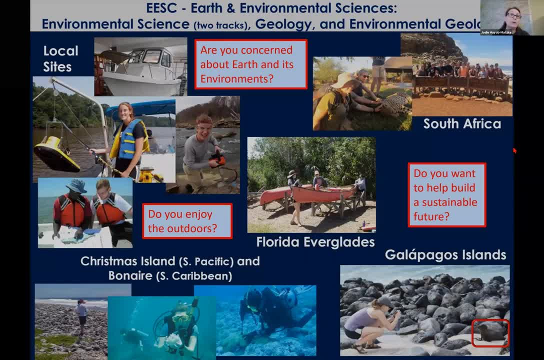 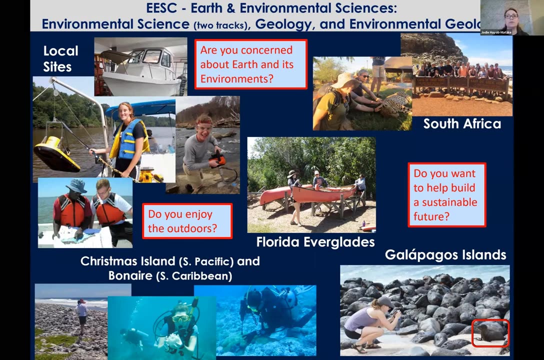 So this first slide is just a fun kind of overview of our programs. My department is called Earth and Environmental Sciences, which is pretty comprehensive and is broad and I think fully encompasses the range of programs that we have to offer. And I'll talk about our majors and our minor in just a moment. But this slide is really just a lot of fun field photographs, to pique your interest in our programs. We have courses that go to South Africa, and Florida and Bon Air and so forth. And these images here show students doing fieldwork in the local region or prior students. So if you enjoy the outdoors, and you're concerned about the earth and its environments, and you want to help build a sustainable future, I think my program or my department is probably a good fit for you. I am Jodi Havmotsky. I'm the chair of the department. 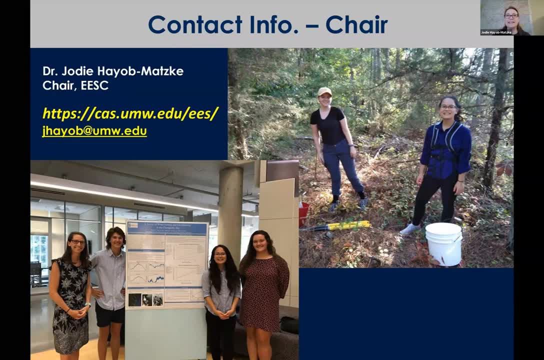 I've been chair for about six years now so kind of getting settled into it. It looks like I'll probably be chair for another term. If you want to reach out to me separately, please feel free to do that. This is my email. And if you forget we can come back to it at the end of the presentation. And then this is a specific link to my department's website and we have a lot of great information on our departmental website. All of our faculty, all of our courses, research experiences, facilities, our rooms and our equipment are all on there. And it's on my email as well so if you don't want to write down this email, or excuse me this website address you can just email me and when I reply to you, you will have a link to our departmental website, as well as our Facebook page we have a Facebook page that's fairly active and that's on my email as well. 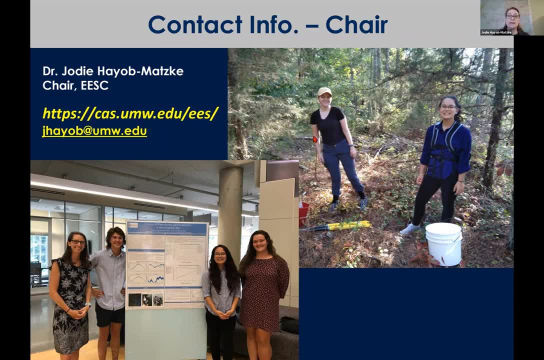 So what you're seeing here is just some of our students. Doing fieldwork in the upper right and then presenting at. This one is actually on campus in the lower left. Let's see with COVID going on will it hinder how far we go or if we take trips at all. 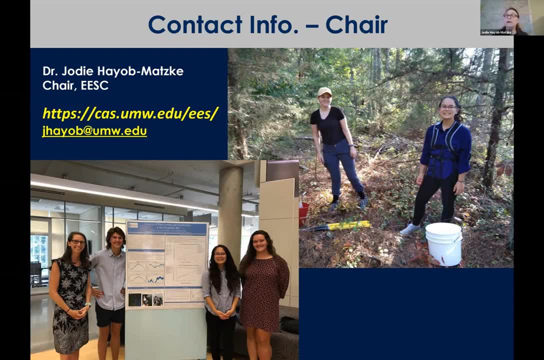 So the plan for next year is to be fully face to face back on campus, assuming that things are normal. We do feel pretty confident and hopeful that by the fall, most Americans will be vaccinated. 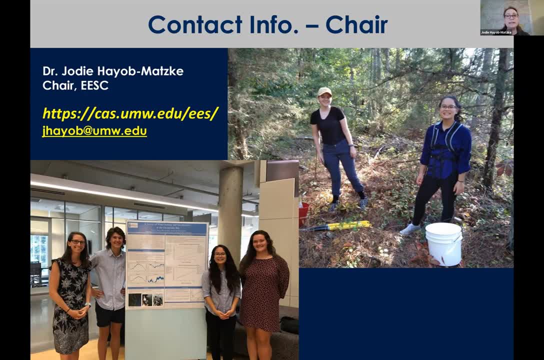 Certainly, the faculty and students. Are strongly supportive of that. And we are anticipating a return to normalcy so we are setting the schedule I just actually submitted the schedule today. 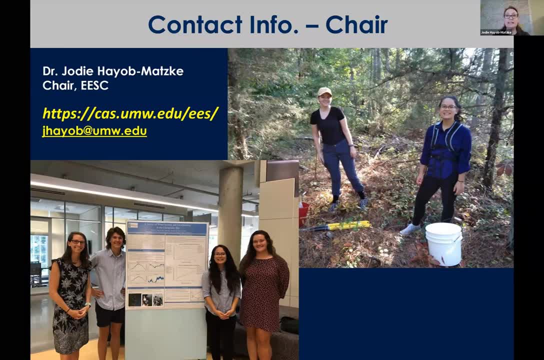 And we are assuming that classes will meet face to face with a lot of field work going on. So that is the current plan. Now obviously something drastic changes over the summer we might have to reevaluate that will be prepared to transition online if we have to, but we're really hoping that that won't be the case. So good question. Looks like there's another one. See. 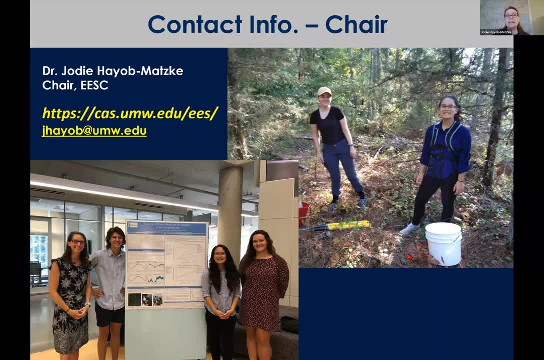 How did I adjust my courses to distance learning. It's been a challenge. We use them quite a bit, like we're doing now and I give PowerPoint presentations at the introductory level. 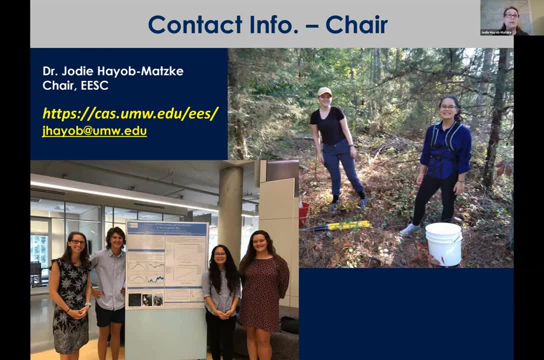 At the upper level, I used a lot of breakout rooms and I put students into breakout rooms because my upper level courses tend to be a block schedule. I don't have separate lecture and lab. So there was a lot of small group work in breakout rooms that I would share handouts with my students. 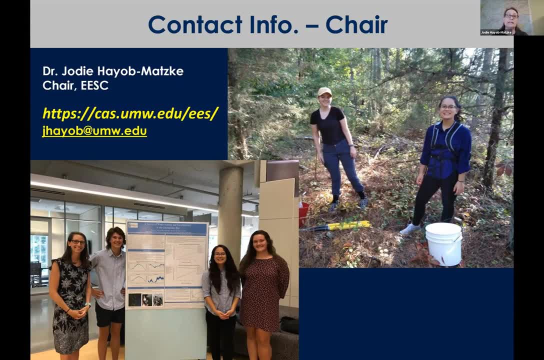 And I actually had my students in my upper level mineralogy class, pick up a custom kit that I created for them last summer so this was a fall class that I taught last fall, and I created a set of rock and mineral specimens for them and some tools like a hand lens and a glass plate and some various things. And so they picked it up at the beginning of the term they met me at the Jepson Science Center. And then we worked together with that identical sample set so that everybody had their own sample set. So that everybody had the same samples. 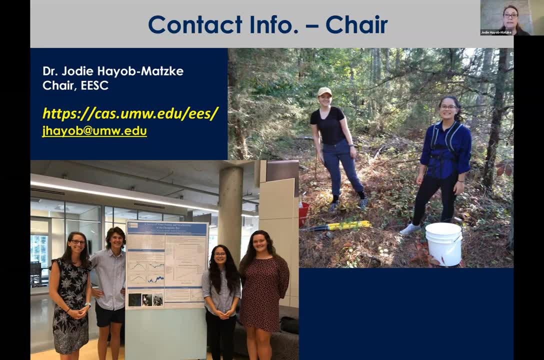 Some of my colleagues did meet students in the field for very localized research based projects. And we did have some face to face or in person instruction with proper social distancing and masking and so forth. I would say that that was more common in the sciences because of the lab component, but it was a real mix probably about 70% of courses total across the university did migrate online. 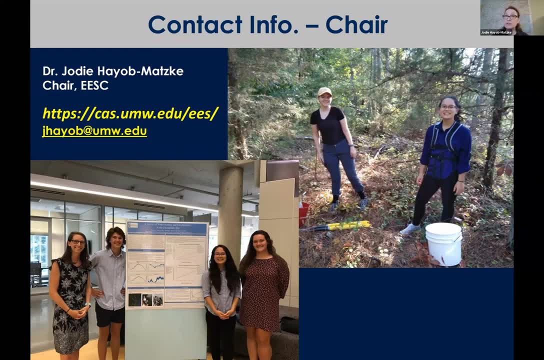 But in the sciences, maybe more like that. Maybe more like 50% so that's a good question as well. 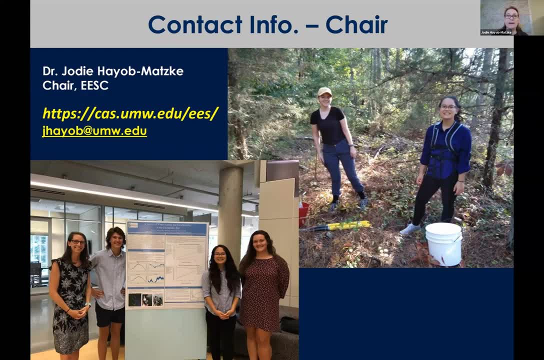 But we all remain hopeful and we do think that by the fall we will be back fully face to face. 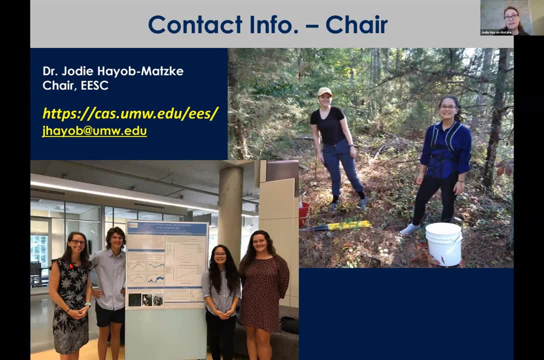 I just wanted to point out in this lower left image that the person on the far left is not a student. Despite her young appearance that is one of our most recent hires, Dr. Pam growth and you'll see more of her in the presentation. 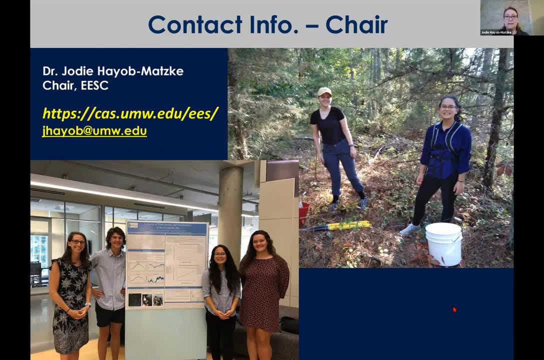 So great questions. Yeah, please keep them coming don't hesitate to give a shout as you have various questions. 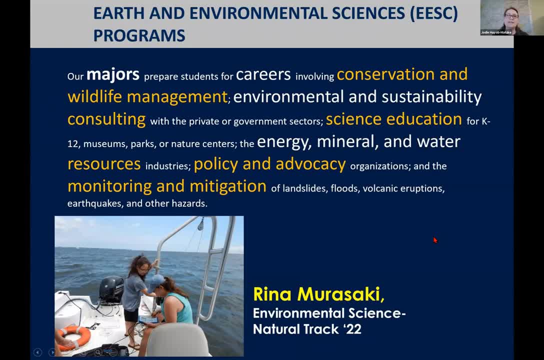 This is more of a marketing type slide that just kind of highlights, some of the careers that students might pursue if they major in one of our programs, everything from conservation and wildlife management to environmental consulting, working in the government or the private sector in education with parks and museums and so forth, but also in the natural resources industry and energy and mineral and water resources is a big part of both geology and environmental science. 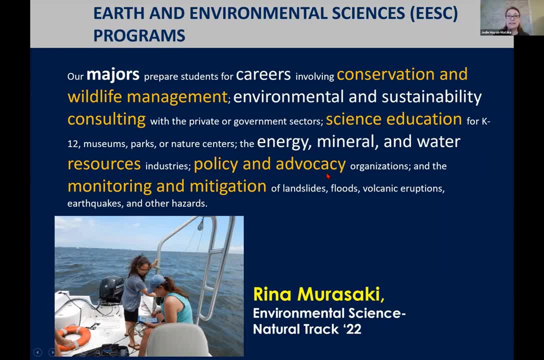 We have some students that like to go into policy and advocacy and work on a variety of issues, such as hazards, like landslides and flooding and so forth, one of our former students works with FEMA in the mapping of flooding, flooding and one of our current students or excuse me former students who graduated a couple years ago and then completed her masters in volcanology works with the Smithsonian, with their volcanology project. This is a photograph of a couple of our students. This is a photograph of a couple of our students. 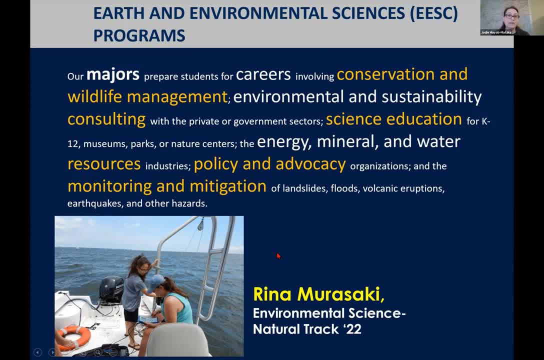 Rena is the one you can really see here, and she's an environmental science major and we do have a 22 foot center console research boat so several of my colleagues, go out in the lakes and streams and rivers and the Rappahannock and the Potomac, and they do field work and they collect sediment samples with the boat. 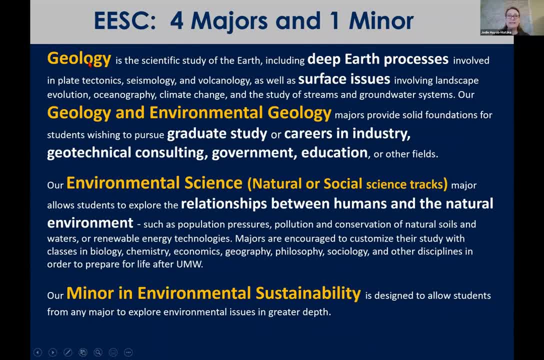 We actually have four majors and one minor. So it's a lot. We have two separate geology tracks. We have kind of a straight geology major. And then we have what we call environmental geology. And that's simply a little bit more focused on surface processes, things like soils, groundwater surface water, that sort of thing. So it's really more targeted to someone who wants to work in environmental consulting. And then we have two separate environmental science majors, one that we call natural science and one that we call social science, and they're both a very strong science basis we don't actually have environmental studies. 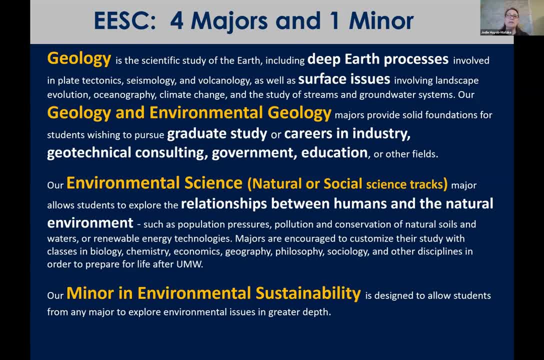 The social science just has more sociology geography economics in terms of elective courses. And then the natural science track the elective courses that students would take would be more within biology chemistry geology environmental science. 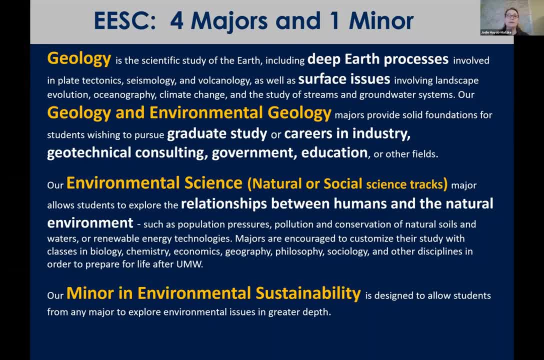 There is a slight difference in the core requirements as well and we can certainly discuss that if people have questions, but they are both basically a very strong science foundation. And then we also have a minor in environmental sustainability and this is really designed for any major. We have at any point in time at least 50 minors, and they take a variety of courses in our program, as well as other departments. So we have certain coursework in geography, even in Spanish and political science courses that are more sustainability focused that can count as electives in the program. We have business majors we have history majors. Geography. Geography majors, geology majors our own environmental science majors, completing this minor so it's a very popular minor and I think it's a very strong program. So let me just pause there for a moment and see if anyone has any particular questions about our majors, or our minor or anything that I've said so far. I don't want to do all the talking but I, but I will. 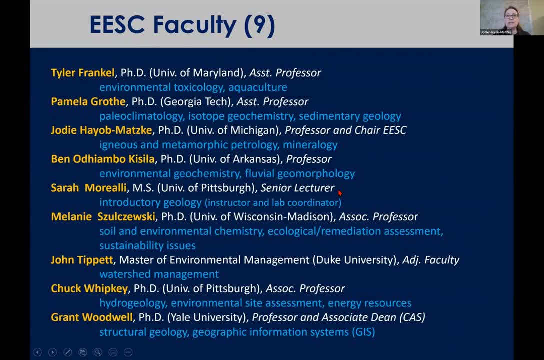 We have nine faculty and this includes Sarah Morelli who is a senior lecturer. So she's an ongoing full time faculty member, just not tenure track she primarily teaches introductory courses, and manages a lot of our lab equipment. And then john Tippett is an adjunct faculty member but he's a long standing adjunct. He's been with us the whole time I've been chair. He has a master's from Duke University and he actually teaches both introductory and upper level courses. He has a master's from Duke University and he actually teaches both introductory and upper level courses. He has a master's from Duke University and he actually teaches both introductory and upper level courses. 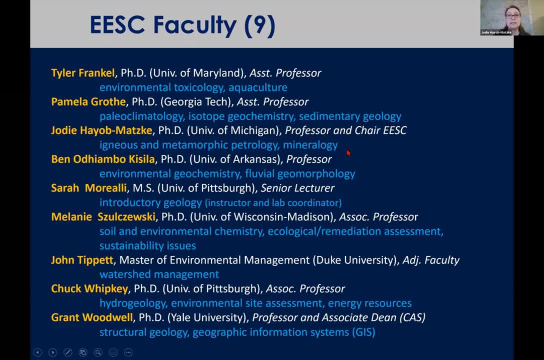 And then the rest of us teach both introductory and upper level courses. 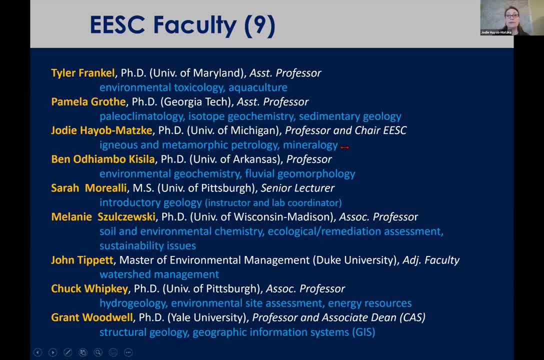 So the question is, do, do we have contacts with the local conservation officer. The short answer is yes, I am a hard rock geologist by training so I am chair of the department. But when students want to engage with the local community in terms of environmental advocacy. 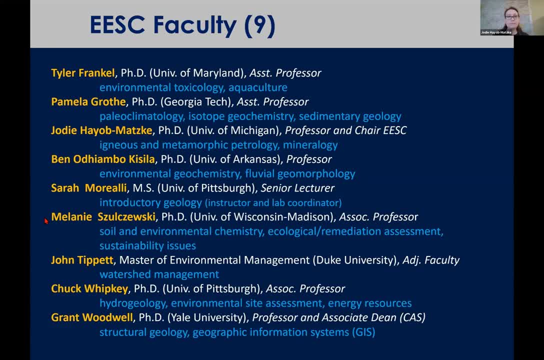 I recommend that they consult with Melanie Schell Chesky, who is one of our non geologists. She does not have a degree in geology. 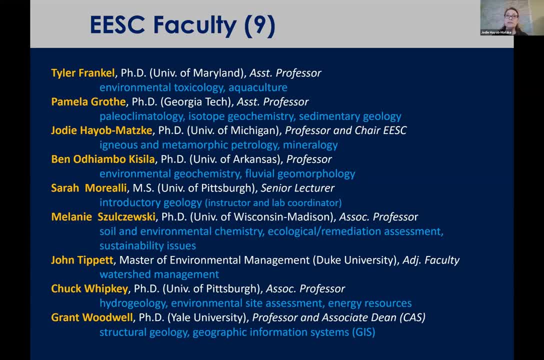 She has a PhD in soil science from Madison, Wisconsin, and she's done a lot of work with NGOs and advocacy groups and actually lives in D.C. and engages a lot with organizations up there. 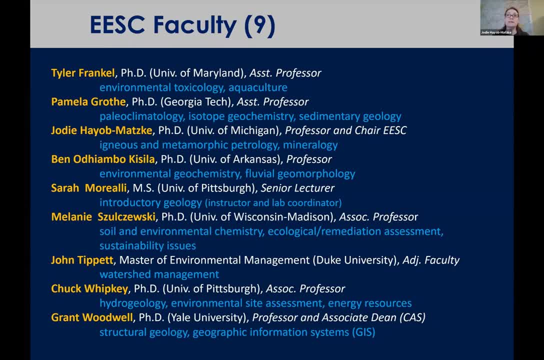 And then John Tippett is actually the former director of the Friends of the Rappahannock, which is a local river advocacy group. 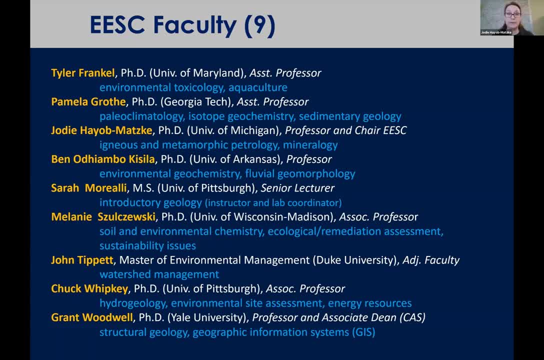 And so he has a lot of great contacts as well. And so do some of my other colleagues. 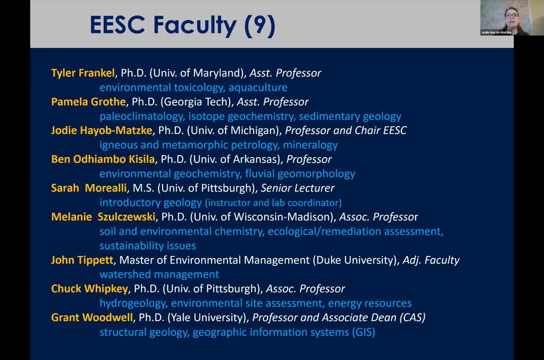 It's just that these are two faculty that I would highlight as being especially well connected with conservation officials in the local and regional community. So I hope that answers your question. If it doesn't, just let me know. 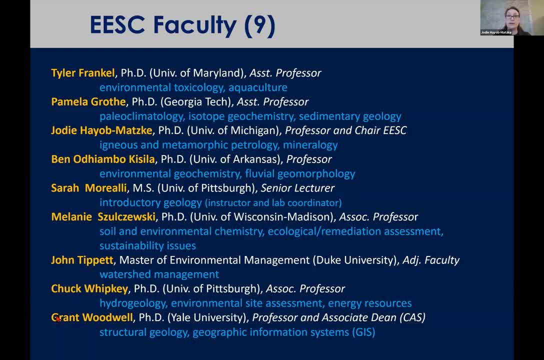 I would also point out that my colleague here at the bottom, Dr. Grant Woodwell, is the associate dean for the College of Arts and Sciences. And so that's been very helpful to have a departmental member kind of in the administration. 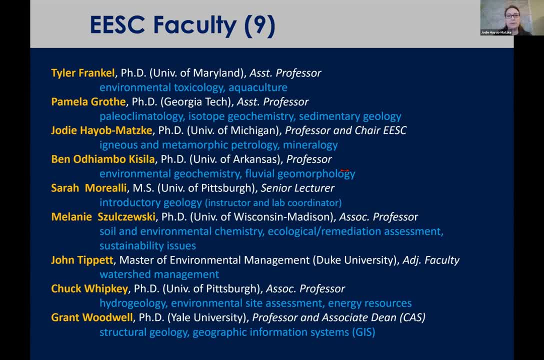 So the question is, what is the closest related program to environmental or sustainable architecture? 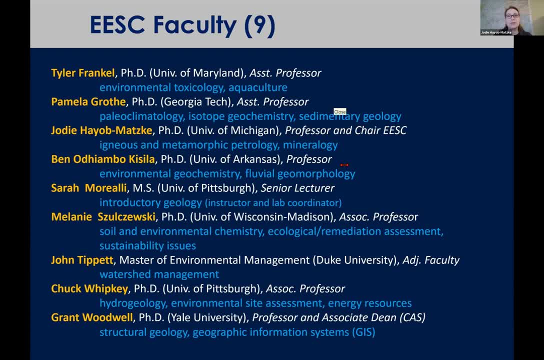 That's a good question. I would say that at Mary Washington, the closest thing to that would be the historic preservation major. 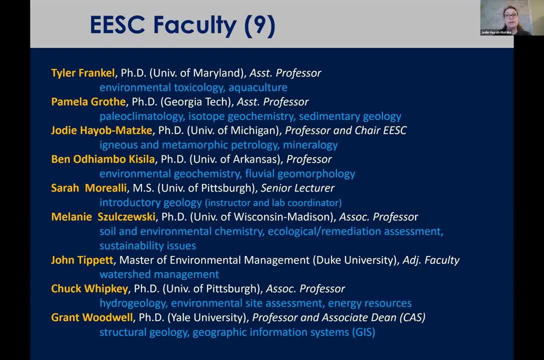 Mary Washington's pretty unique in having an undergraduate degree in historic preservation. And there aren't that many universities in the country that specialize in historic preservation at the undergraduate level. 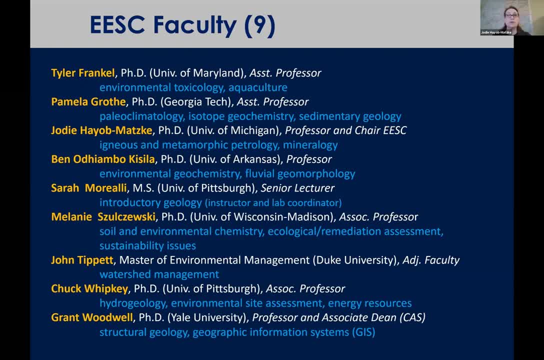 So if you have interests in those areas, you really should check out historic preservation. It's a great program. 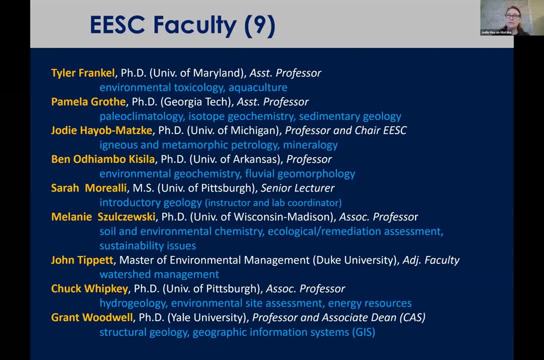 And maybe consider a double major or a sustainability minor with a major in historic preservation or something like that. 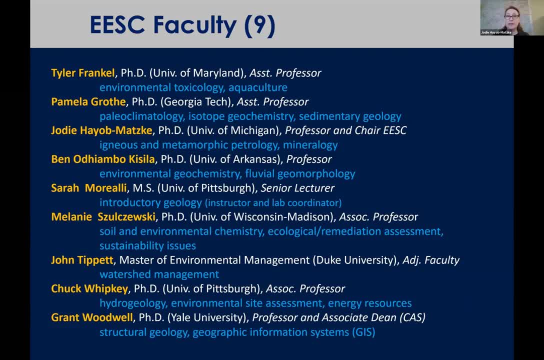 And if you email me at the end of the presentation, I can put you in touch with the historic preservation folks. 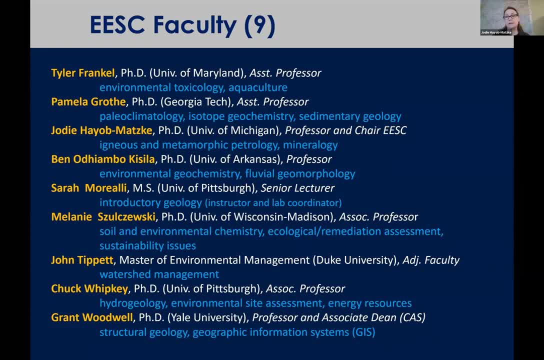 Or you can look on the Mary Washington website and search under academics, and you should find them pretty readily. 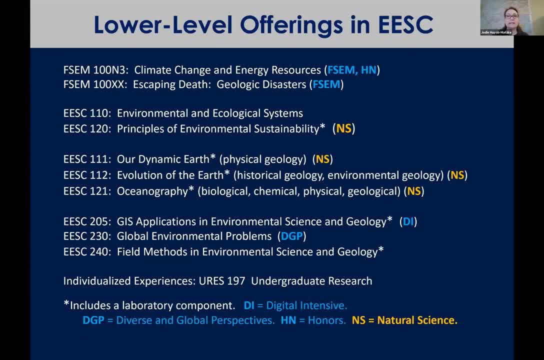 We have a variety of lower level offerings, and I've simply flagged in terms of like gen ed purposes. 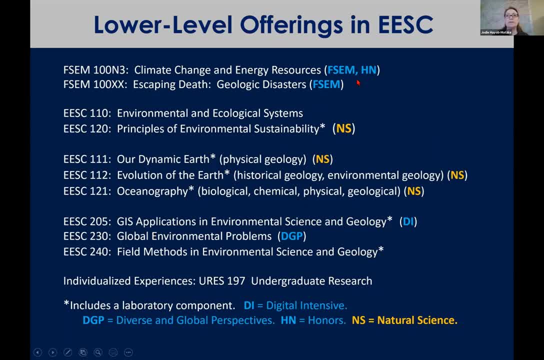 Which of our courses would count in certain areas. So we have a couple of freshman seminars or first year seminars. We have these two courses here. The 110, 120 is essentially the year of introductory environmental science. The NS means that that particular course satisfies the new general education natural science requirement. 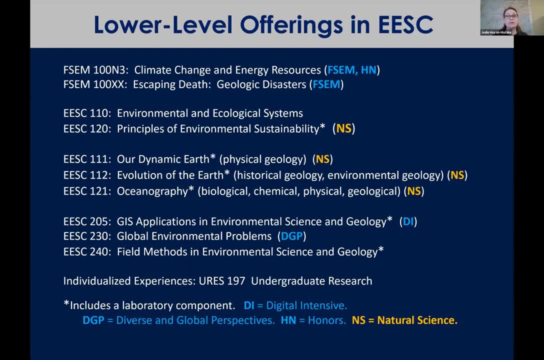 The 111 and 112 is essentially the year of introductory geology, what a lot of schools call physical and historical geology. And then we have an oceanography course as well. 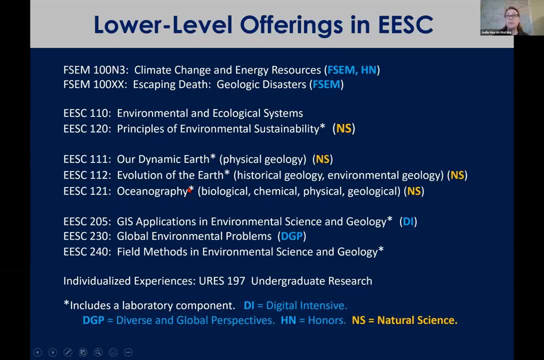 And any of these courses that have the asterisk are for credit lab based courses and therefore satisfy the natural science requirement. 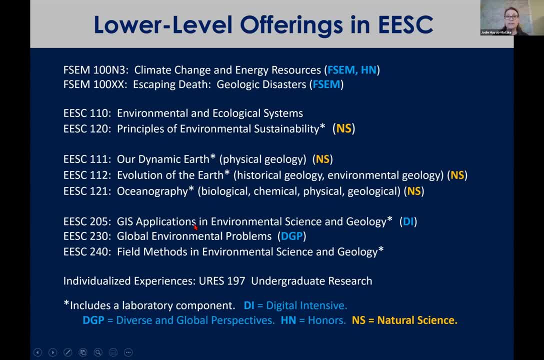 We do have a GIS class that my colleague Grant Woodwell teaches, and it counts for the digital intensive general education requirement. 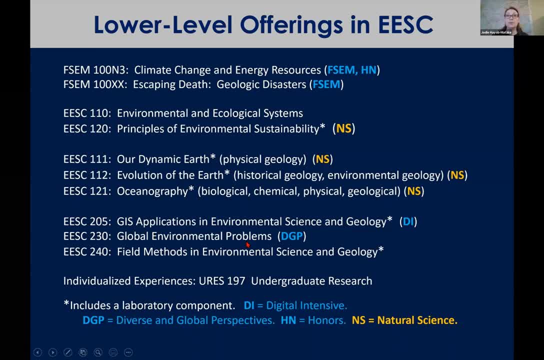 And then the adjunct John Tippett that I mentioned teaches our global environmental problems course, and that counts for the diverse and global perspectives, which is a general education requirement. As well. 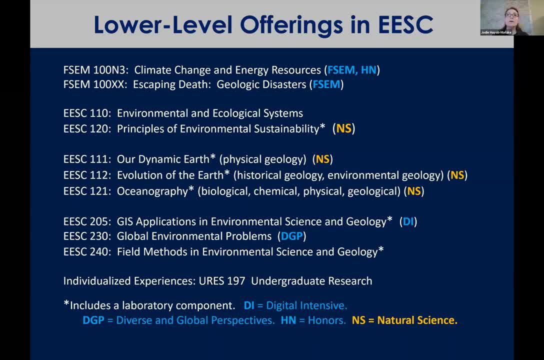 So the point I'm making here is that by doing a major in one of our programs, you can get a lot of the required or a fair amount of the required general education requirements as well, and kind of double dip in that regard. 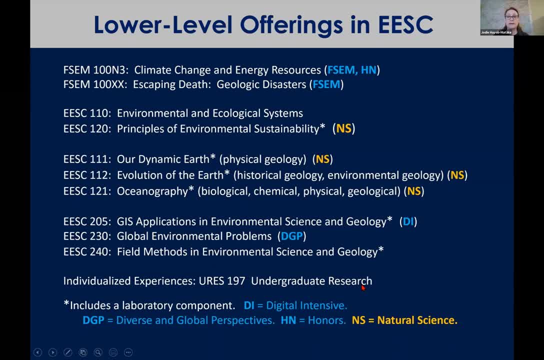 We have an introductory field methods course, and the US 197 is something that's offered in virtually every department at Mary Washington. 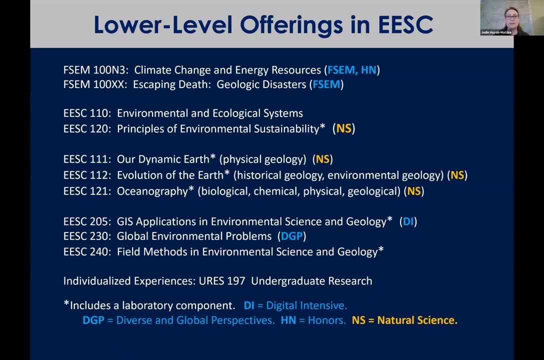 So these are just the 100 and 200 level courses. And if you have any particular questions about any of these, I would be happy to answer those. I don't know how many students are familiar with GIS. 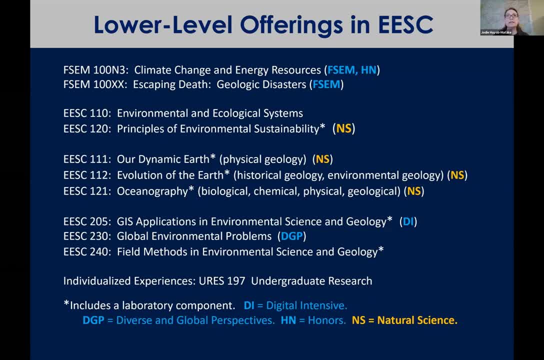 GIS stands for geographic information systems. It's essentially digital map making. So if you've ever visited a website, and you've pulled up data that had a spatial component or an aerial distribution and you've clicked on features on a map like I think most people have, this is essentially what GIS is. 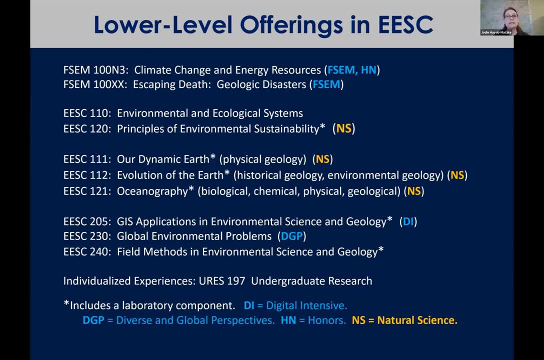 And Mary Washington was one of the first, I think the first in the state of Virginia, to do this. And she was one of the first in the state of Virginia to offer a certificate in GIS. And it's a series of five courses, and at the end of that, students are certified with this GIS certificate. 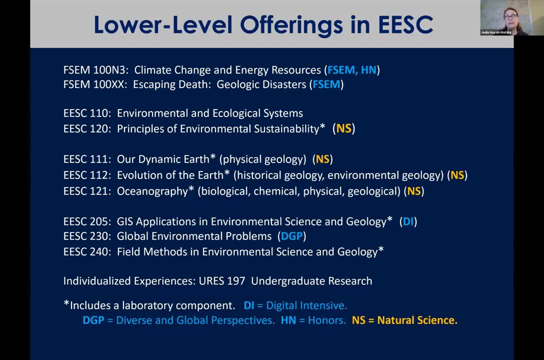 So it's not a minor. I would say probably upwards of 20 to 30% of our majors complete the certificate, because I think you would be very hard 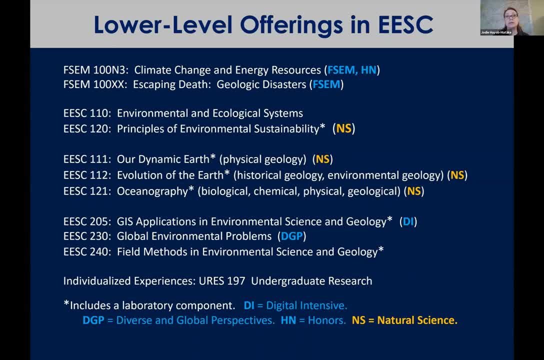 pressed to find a job in environmental science or geology that doesn't require strong GIS skills. It is really the wave of the future. It's pretty expensive. 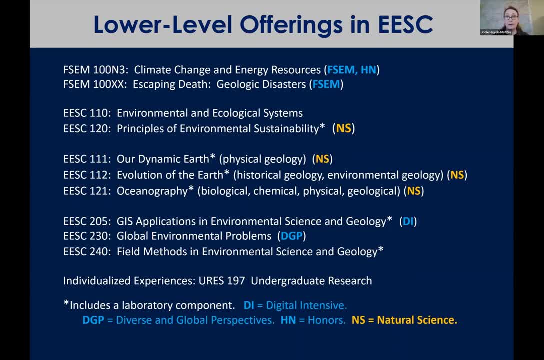 It's a pretty essential, a pretty essential toolkit to have. So all of our majors require students to take an introductory course in GIS. 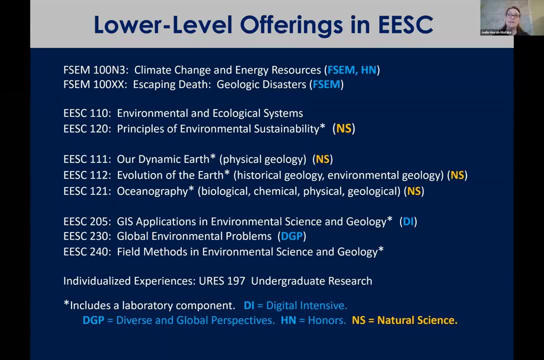 And then with an additional four courses, some of which count as electives in the major, you can get the certificate. So it's a pretty popular thing. 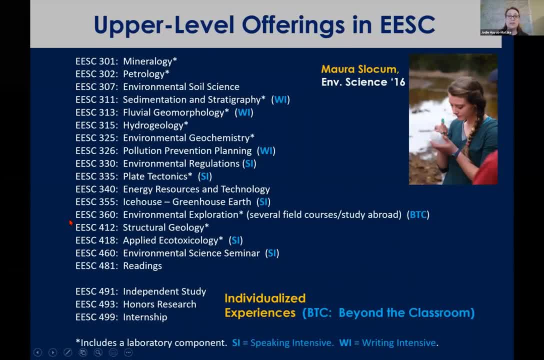 We have upper level courses, too, as well. I've simply listed these in numerical order. And again, the ones that have the asterisk next to them are lab-based, four credit courses. 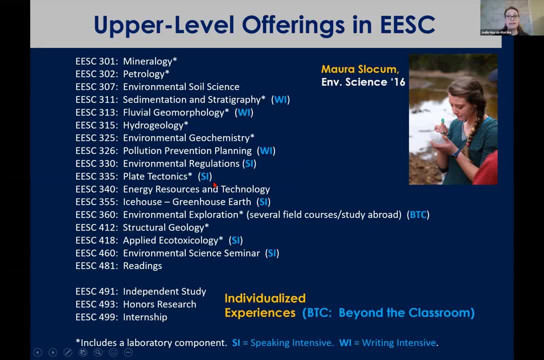 The SI are writing-intensive courses, and the SI are speaking-intensive. Let's see, there's a question in the chat. 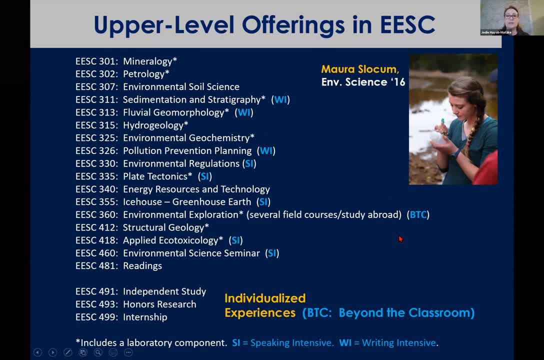 How quickly is the GIS certificate program completed? So it's a series of five courses, an introductory GIS course. What's the next one? Spatial problems, I think it's called. 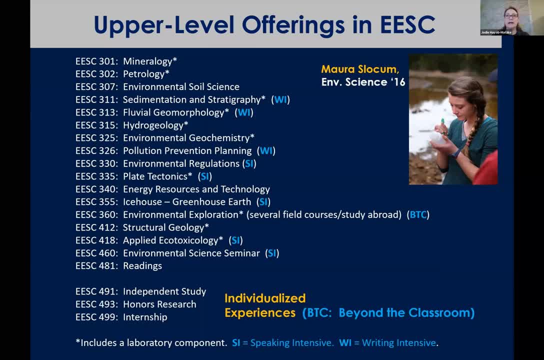 There used to be a programming requirement. They may have taken that out. 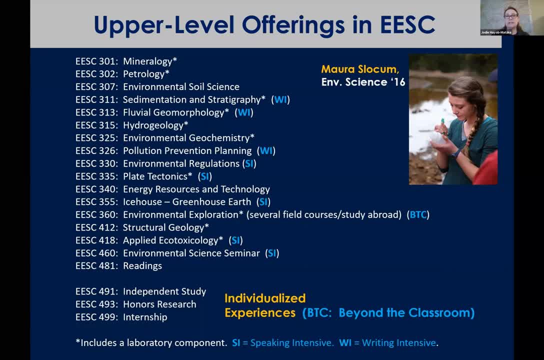 Then you choose one elective. And remote sensing, for example, which is a popular course that our students would take, is one of those electives. 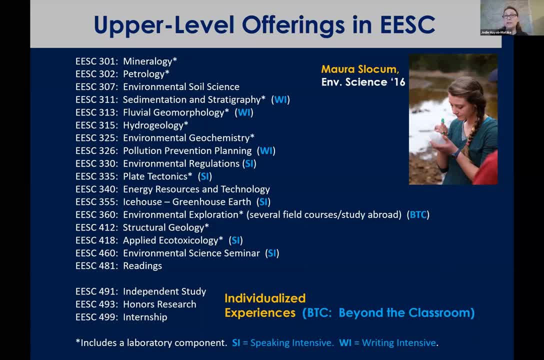 And then you do a capstone experience, either research or an internship. And that's a great foot in the door for a job. 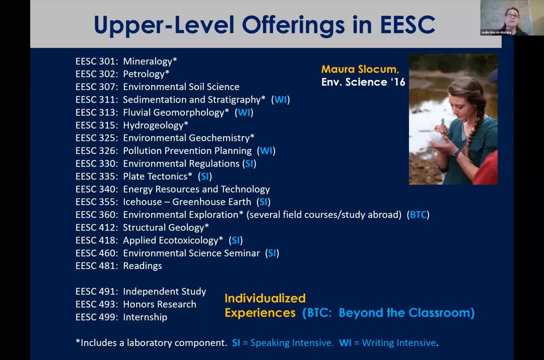 So it is a certificate program that is designed to be completed by any major. And I would say that if one took a normal course load and then was interspersing some GIS classes, you could easily get done in two years. 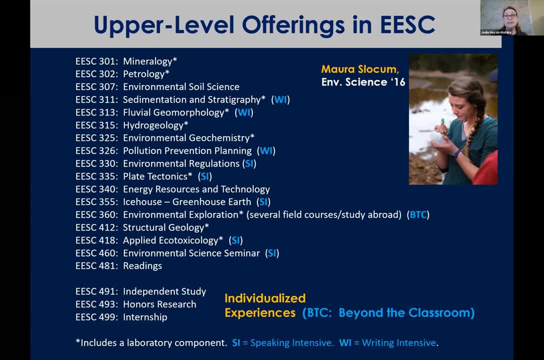 And if you simply just wanted to get the GIS certificate, you could do all of that coursework in probably a year and a half, if not maybe a year. 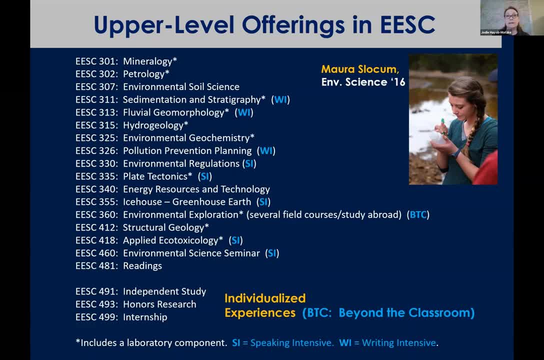 And some of those courses are offered at night and in the summertime as well, because they're really intended for the general public as well. There are people from the community that have completed that certificate, not just our own students. So it's a really popular thing. It would not be a difficult thing to complete a major and do that certificate. So it's a great thing. 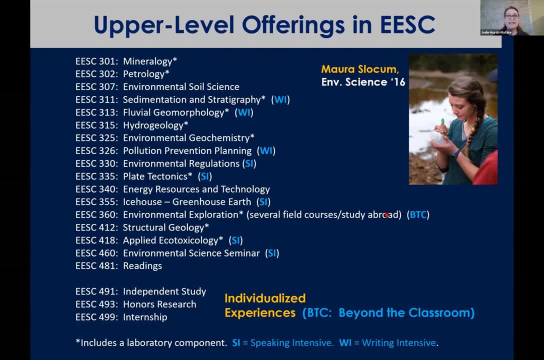 kit as well. I see more questions. Good. Do you know if AP capstone research would be able to count for the capstone experience? I'm not sure what you mean by AP capstone research. If you mean like AP, like advanced placement from high school, the answer would be no. This has to be a 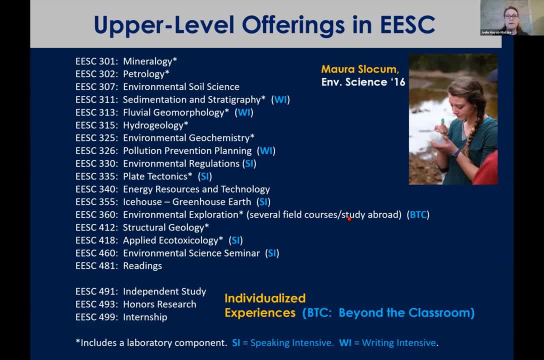 college level experience. But if you mean just any old capstone research, for the GIS certificate, the capstone project has to be GIS related. So that's housed in geography. The Department of Geography houses the GIS program. But we have students in our program majoring in geology or environmental science who do the certificate will typically choose a geological or an environmental science-based research project. And they kind of get double credit. They get capstone experience credit for their certificate, but then they can also count it in the major. 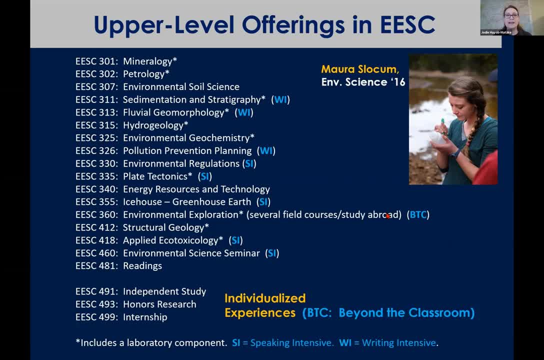 Let me just check the chat again. Oh, I have not said what classes I teach. So I hope, Gabriel, I answered your question. And if you have questions about the GIS certificate program, 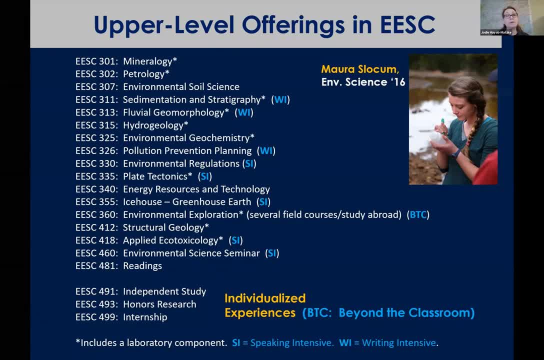 just email me and I can forward your contact information to the chair of geography, Dr. Jackie Gallagher, and she can answer your questions. 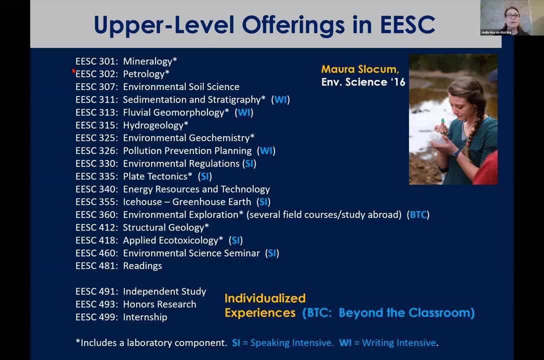 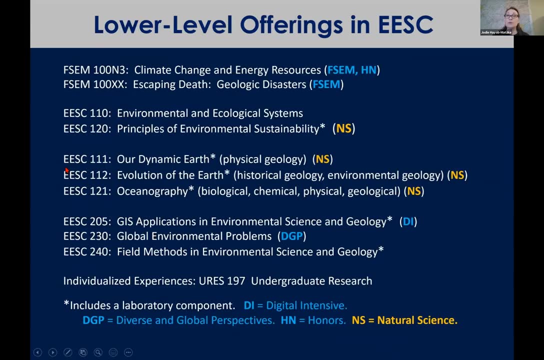 I have not said which classes I teach. I teach the mineralogy-petrology sequence. I am a hard rock geologist by training specifically metamorphic rocks are my specialty. So I teach, if I just go back for a second, whoops, if I can do that. I teach the 111 and the 112, which is essentially 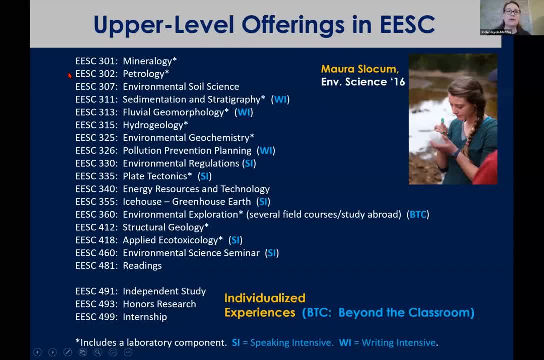 the year of introductory geology. And then I teach the mineralogy and petrology. So a year ago, when we had to go online in the spring of 2020, I was in the middle of my petrology class and we had to migrate online. 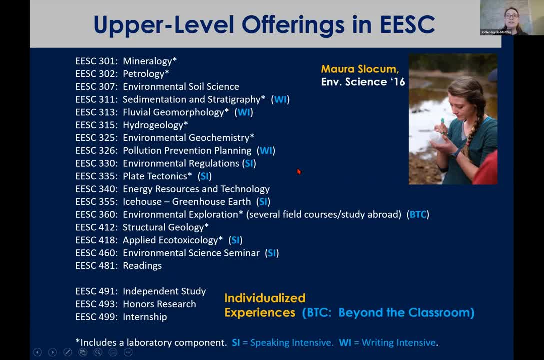 And then I taught mineralogy online last fall. And that was a challenge. I didn't love the lack of being a face-to-face because it's very hard to do microscope work in a virtual setting. So I'm really anxious to get back in the classroom for this coming fall. 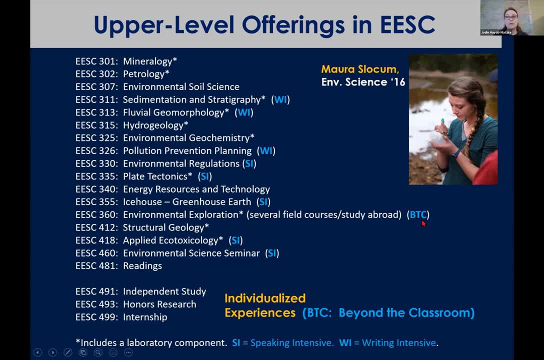 Yeah. So the BTC here stands for beyond the classroom. That is, it's a new twist on an old requirement. If you're not aware, starting in fall of 2020, this past fall, Mary Washington instituted a new set of general education requirements. They're a lot more flexible. We now accept, if you're not in the know, as some students don't appear to be, we now accept four years of the same language in high school that will waive your foreign language requirement. That's been a very popular change. And we now have a little bit of a pared down foreign language requirement. So through the third semester, as opposed to the fourth semester, we now have a little bit of a pared down foreign language requirement. So through the and the science requirement unfortunately changed a little bit too. But one thing that we do require is that every student complete a beyond the classroom experience. And this is really meant to be a more engaging experience outside the traditional classroom. And so virtually every program has courses that count. Certain study abroad programs count for this. Internships, 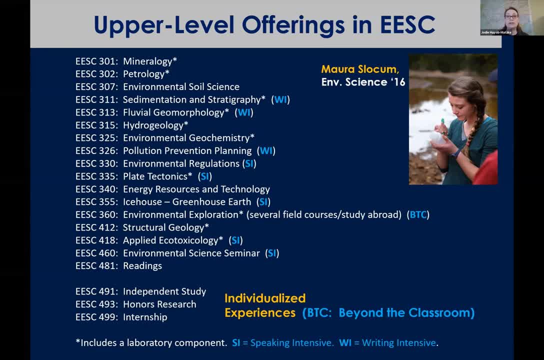 research counts, and as well as service learning projects and so forth. So my department certainly has several opportunities for students to complete that as well. And then every student has to do a speaking intensive course and a writing intensive course in the major. And then there are some additional SI and WI courses required, but at least one of each has to be in the major. So the point to all those little acronyms here on this slide is just to reassure you that you can do that in our majors. That's not going to be a difficult thing to do. 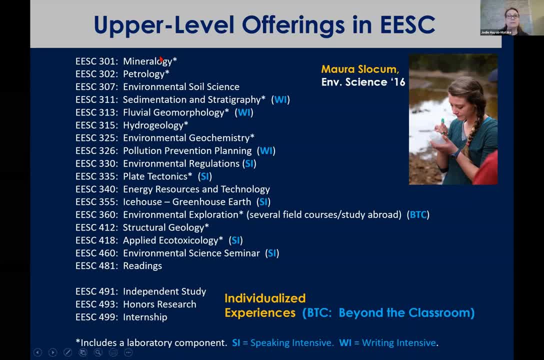 So if you're more interested, in geology side of things, mineralogy, petrology, soil science, sedimentation and stratigraphy, river, landforms, which is what that means, surface and groundwater, environmental geochemistry, environmental regulations, plate tectonics, really all of these. 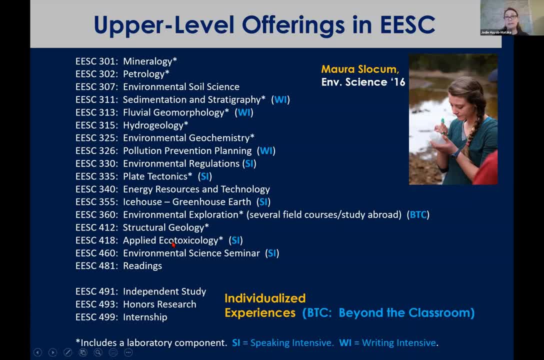 The one thing that may not be of interest would be the applied ecotoxicology. This does have biology required to take this. So we have a fairly new hire who is a biologist by training and he teaches a toxicology course. And that's a really exciting, fun thing. And I can say more about his research as we go along, if you'd like. But for now, let me just pause a moment and see if folks have any questions about the upper level courses that I've listed here. 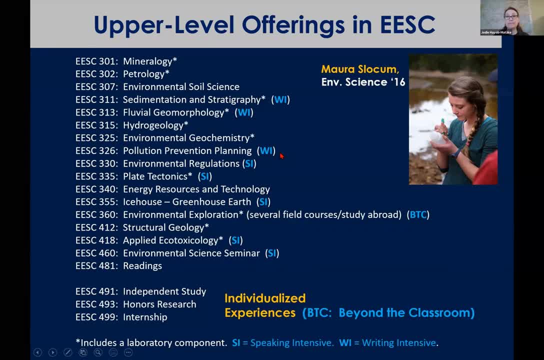 If you don't see an asterisk, it means it's a three credit non-lab course. So we have a mix of both. I think my department more than any other in the sciences has a mix of both three and four credit courses. Most of the biology and most of the chemistry courses seem to be four credits with lab. And we have quite a few that are not, which is really nice for scheduling. It kind of gives students a little bit of a different approach and perspective to not always have so many labs. 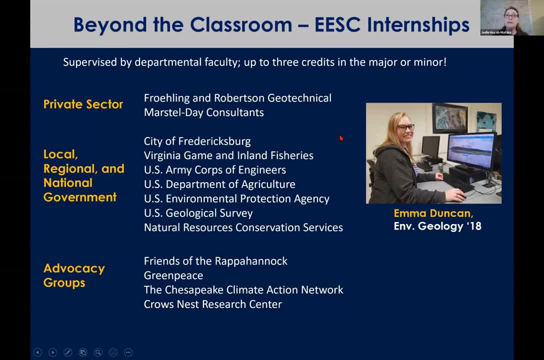 This is just highlighting some of the various organizations that students have interned with. The private sector, these are both private environmental consulting firms. Local, regional, and national government, including the U.S. Army Corps of Engineers, the USDA, the EPA. This is the federal EPA up in D.C. If you didn't know, at the federal level, the United States Geological Survey, the headquarters are just up the road in Reston, Virginia. So that's really nice. 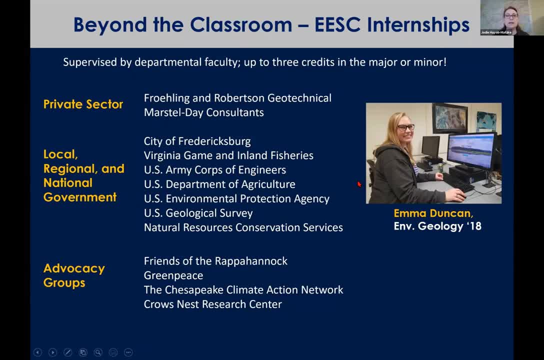 So what is the difference between three and four courses time-wise? Do you mean between three and four credit? Like a three-credit course versus a four-credit course? Yeah. And then I'll tell you about Tyler's research because that was another question in the chat box. A three-credit course typically meets for three hours per week, either Tuesday, Thursday for an hour and a quarter or Monday, Wednesday, Friday for 50 minutes. And that's it. So the contact hours are what we call three hours per week. And that's it. So the contact hours are what we call three hours per week. 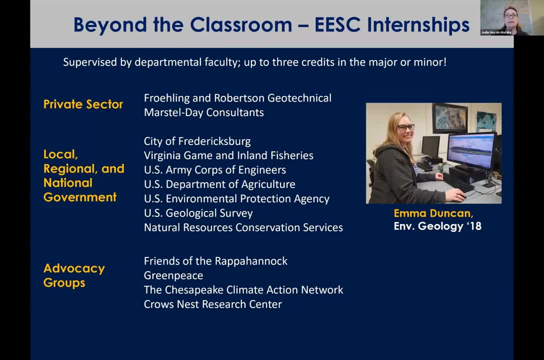 Four-credit courses are a lot more work. They actually typically have six contact hours, even though they're only four credits. So that one credit of lab is really like three or four contact hours per week. You have the three hours of lecture and then typically three hours of lab. So in my department, all of the upper-level courses that are four credits, almost all of them, yeah, all of them have six contact hours per week. So you can start to see how that really factors into the workload. I would say that students in the sciences tend to take between 12 and 15 credits per semester, sometimes 16 credits. So sometimes it's three courses. Sometimes it's four courses. If you're taking several labs, you probably would not take more than four courses at a time. Yeah. And then, 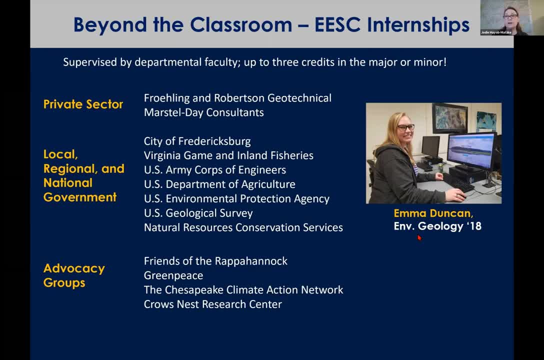 so this is Emma Duncan who graduated a couple of years ago. She was an environmental geology major and she's working on a GIS project. And then this is Friends of the Rappahannock. This is that advocacy group I was telling you about. And then this is Emma Duncan who graduated a couple of years ago. She was an environmental geology major and she's working on a GIS project. And then this is Friends of the Rappahannock. This is that advocacy group I was telling telling you about that John Tippett was the former director of, and these are just some other advocacy groups that our students have interned with. So the Friends of the Rappahannock and the Crow's Nest are more local. Greenpeace, of course, is a national organization. So a range of scales here. I'm going to show you a slide that highlights some of the research projects. So I will come back to the question about the ecotoxicology research. I promise I won't forget that. 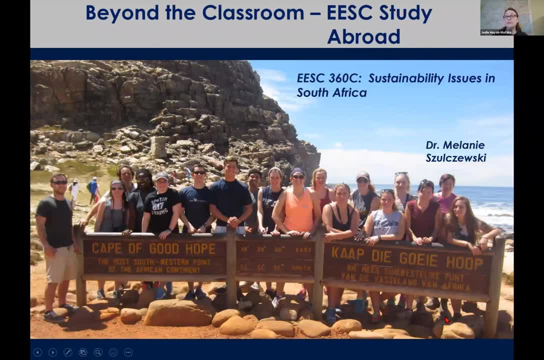 All right. I just want to highlight a little bit about some of our study abroad courses. 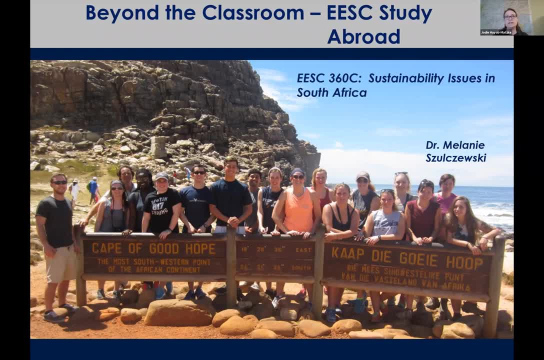 Mary Washington has really made a lot of changes, I would say, over the past five years. 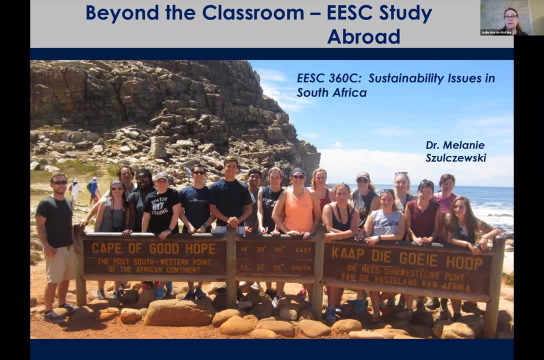 If you go to the Mary Washington website and you just search under study abroad, we have a CIE or Center for International Education, and we have a lot of study abroad courses. And if we don't offer them, we partner with other universities. So students can go to one of our partner universities and take coursework. And if they don't offer them, they can do a semester abroad and then transfer it back to Mary Washington. And you know that it's going to count, and you know in advance what the courses are going to count for. This is my colleague, Melanie Shulcheski, right here, who every other year leads a course to South Africa. 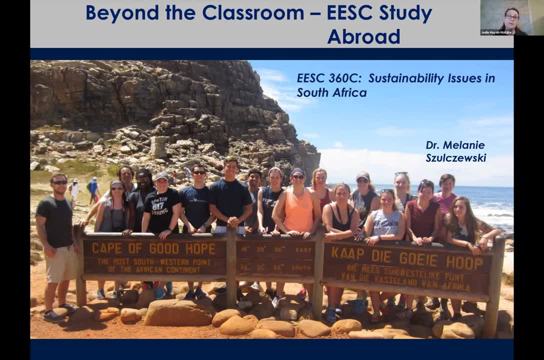 She worked in Cameroon in Africa in the Peace Corps a number of years ago. So she's had a lot of experience working in Africa and volunteering. 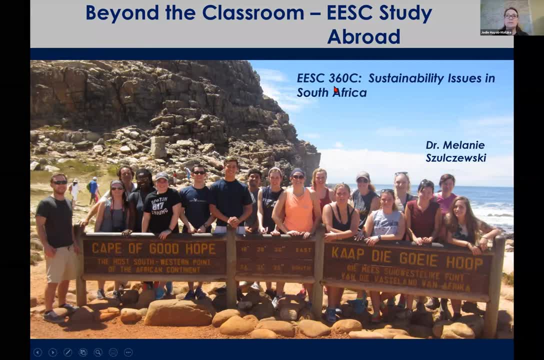 And so we have a course called 360, which I think the title is just Environmental Exploration, but then it's the letter that tells you which specific course. And so this particular course is called Sustainability Issues in South Africa. It's a four-credit course where students go to South Africa for two weeks in late December. And then in the following spring, they do the classroom component of the course. And so there are extra fees, associated with these study abroad courses, but the tuition is not any different. The tuition is 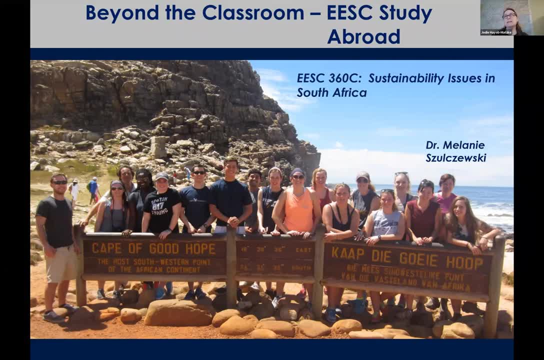 embedded into your normal spring course load. So you would be taking this as a four-credit course in a particular spring semester. And in that regard, you don't pay any extra tuition. It's part of your normal load. But Africa is not a cheap place to get to. So the flight and the 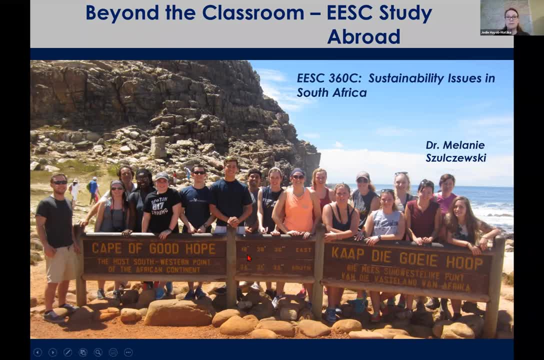 room and board while you're there does have an extra cost. And this is them at the Cape of Good Hope with the class that she took. 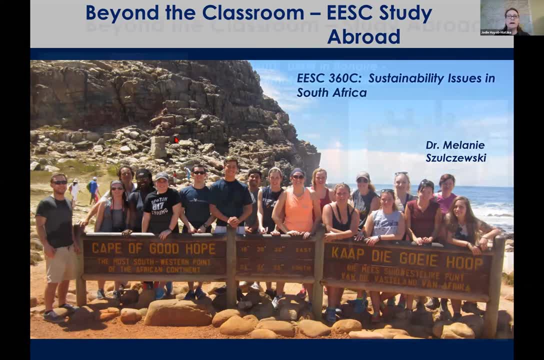 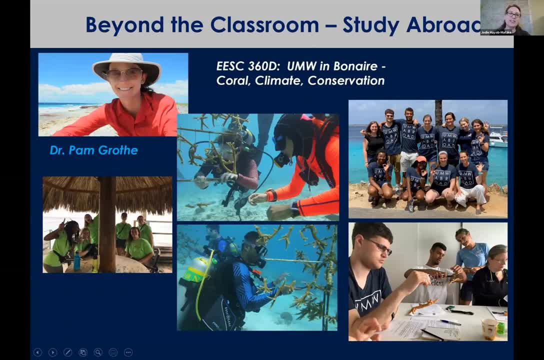 My other colleague, Dr. Pam Groth, who's actually an alumna of Mary Washington, 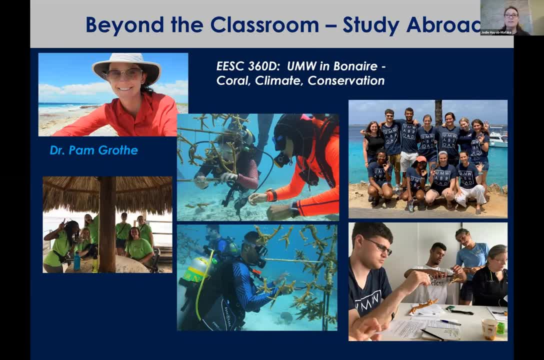 she graduated in 2006 with a degree in geology. And she was so good. We hired her a couple years ago. She's our second to most recent hire. And she developed this course in Bonaire on coral, 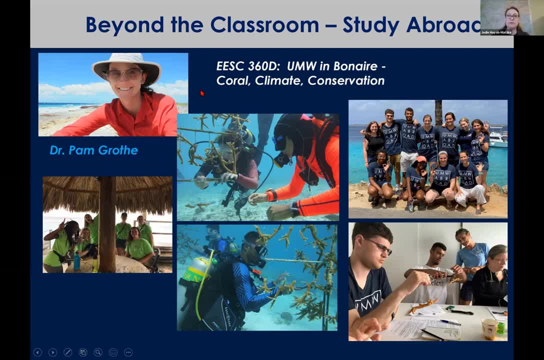 climate, and conservation. So Pam is a climate change expert. She uses fossil corals to study research. And she's a professor at the University of California at the University of California. 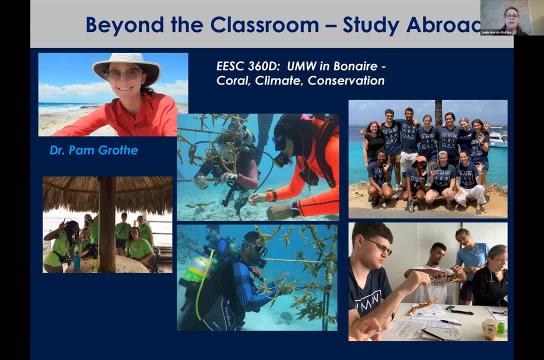 She's a professor at the University of California at the University of California. And she's a professor at the University of California. And she's a professor at the University of California. So she's a graduate at the University of California. And she's a professor at the University of California. And she's a climate change over the past 10,000 years or so. And this is a course where students go to 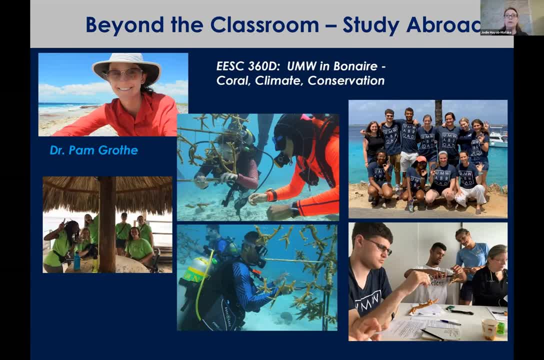 Bonaire over spring break. And they would take this four-credit course during the spring semester when it's offered. And then the field component, the one credit for the lab is this week in 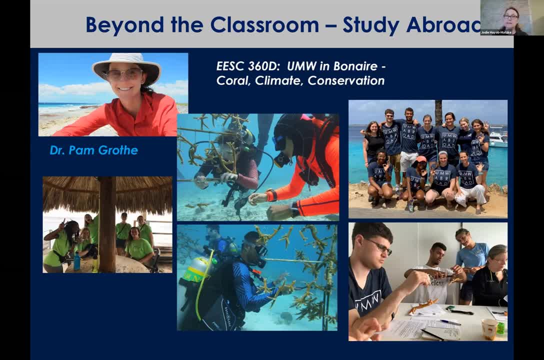 Bonaire. And again, it does have extra costs associated with it. 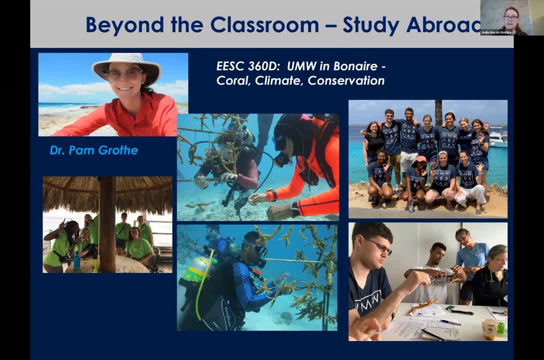 her and a little socialization there as well so we'll meet there a moment 30 or just 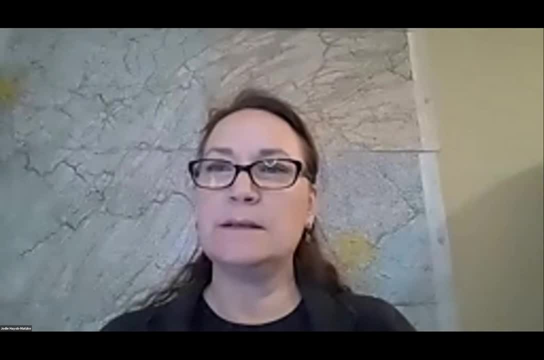 all right i can't tell if i'm muted can you guys still hear me kelly yeah okay sorry i got this weird people trying to log on message 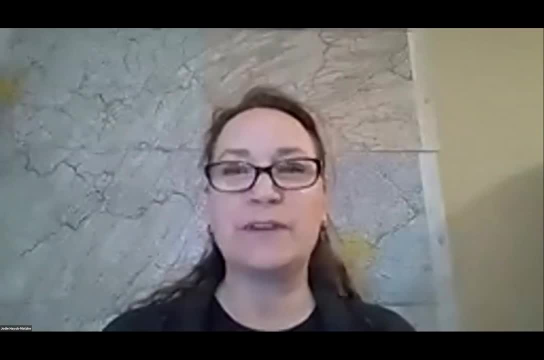 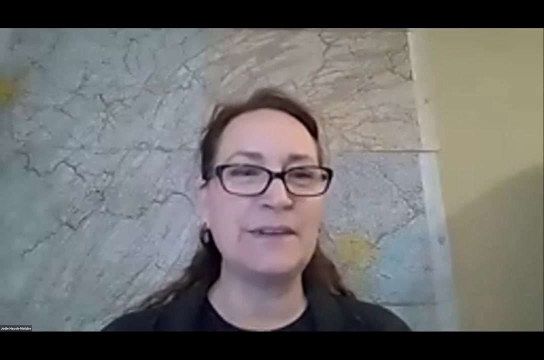 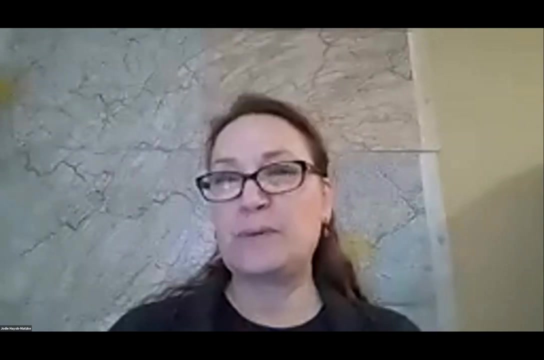 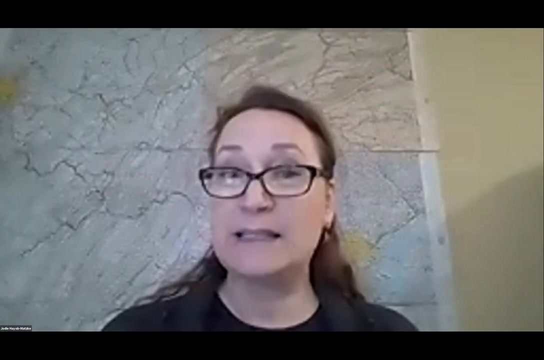 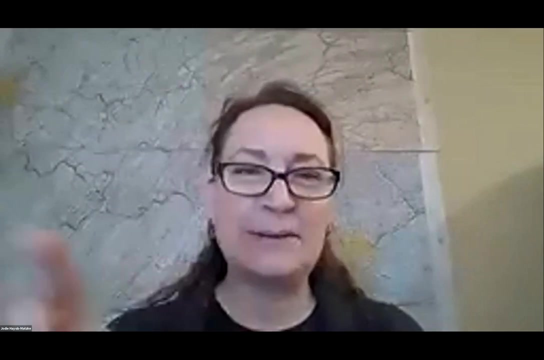 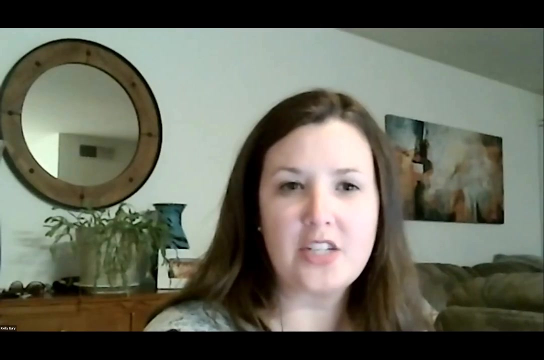 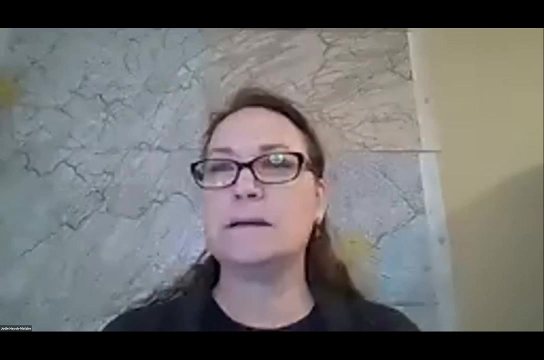 that you had muted folks all right uh we also have a florida everglades course this one has not been run as recently because mel and pam developed these other courses and our students seem to like to go abroad more so than down south but this is melanie in the field doing some things and students going canoeing uh and some giant tree i don't know what that is but this is another 360 course that we offer i'm getting a message that my internet connection is unstable so if you can't hear me please let me know i can hear you jody but kelly i can see you in the little um we lost your shared screen we lost your presentation oh okay okay let me um end the show and let me see how to get back to that okay i look hot so this is uh yep so everyone one person back just anyone who is sharing i have referred to a blackboard to be able to get that to me why's chat 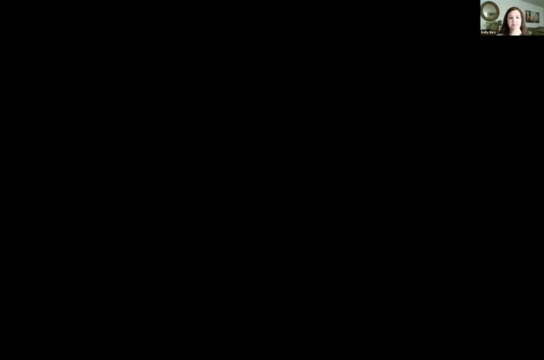 do you know how far back you lost that 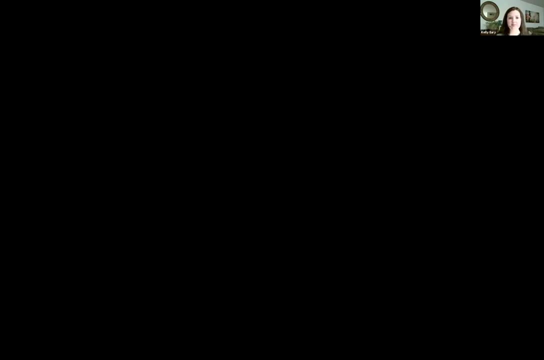 we were you were on with can again okay 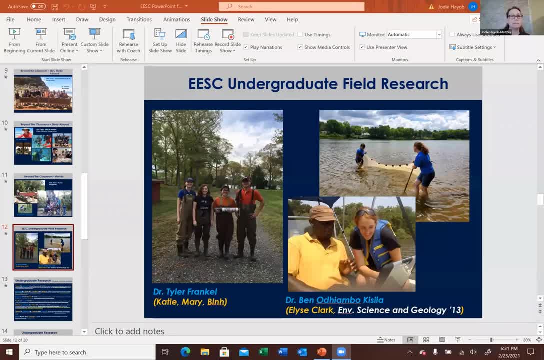 oops one more was i on this slide um it was the one with pam when she was in bon air pages i cushioned her this video is full of greenery i didn't know how to limit my time holding herرف 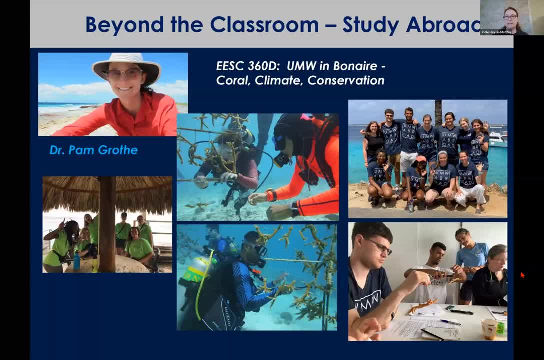 Yeah. Okay. Sorry about that. Technical difficulties. So yeah, Dr. Groth has this new course, fairly new course that she takes students to bond there. Did you hear most of what I said or did you hear me speak for a while on this slide? Yes. Yeah. Okay. All right. So I think what you probably missed was this slide about the Florida Everglades and how Melanie 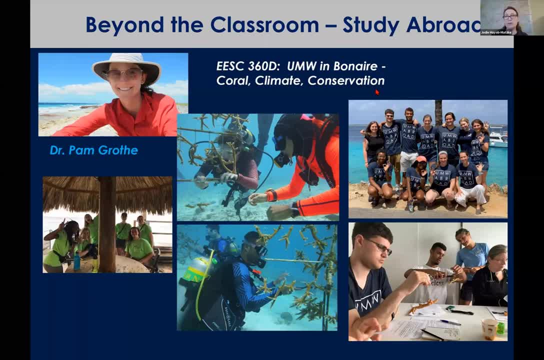 Schultesky and my colleague Chuck Wipke in the past, this was actually the first, that's why it's 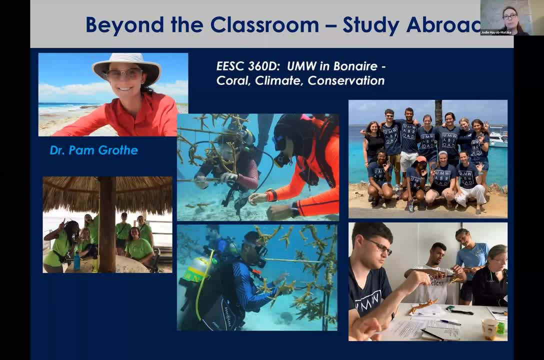 A, the first 360 study abroad, not really abroad, but field-based course. And they haven't run this 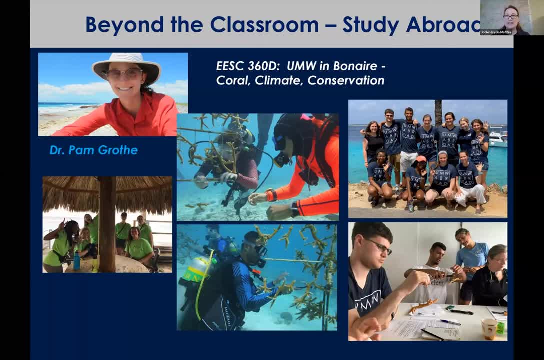 one in a while because these other more exciting locations have been developed. But this is many 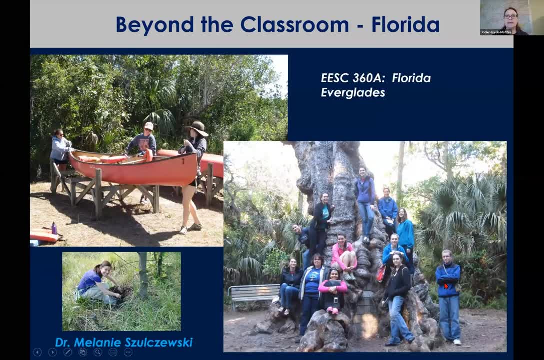 students in the field in Florida. And then I think I was getting to this slide when I 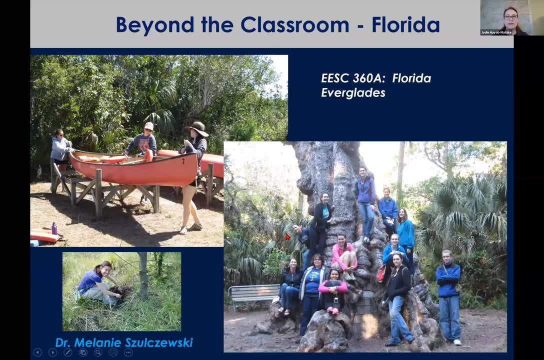 booted out. This is Dr. Tyler Frankel. This is Dr. Ben 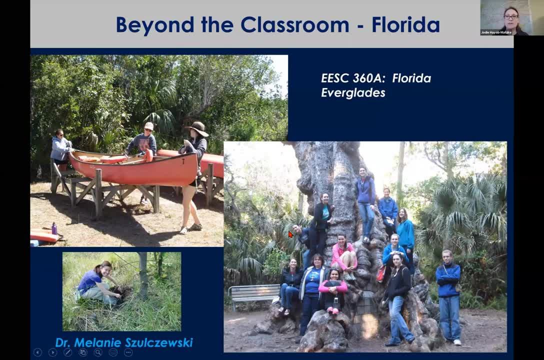 Odeombo-Casella and with some of their students doing field work. This is Ben and Elise Clark was 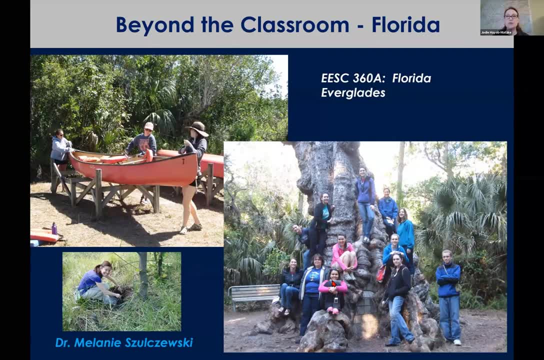 an environmental science and geology major. She was a double major back in 2013. And she's now 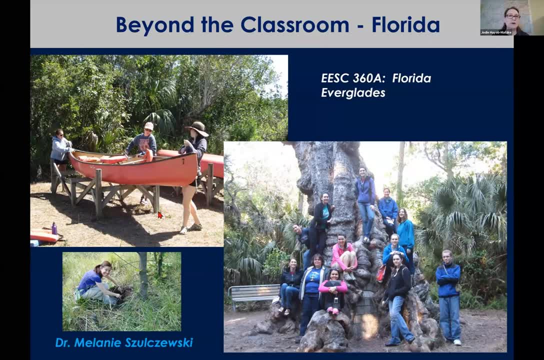 an assistant professor at Fitchburg State University. So that was, she graduated almost eight years ago. And then Ben and Mary and Katie. Katie is a current student and these two graduated 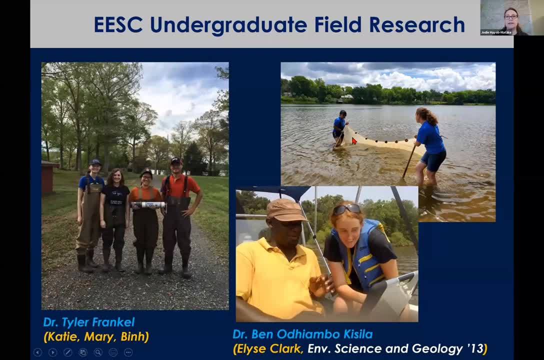 last spring. And so this is Mary and Ben collecting, I don't know what they're doing because I'm a hard rock geologist. 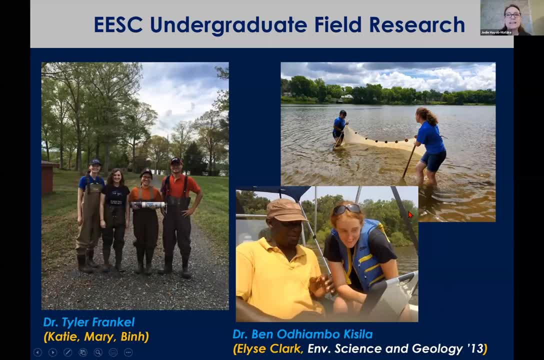 But they're doing something in the river. Let's see, there's another question in the chat. 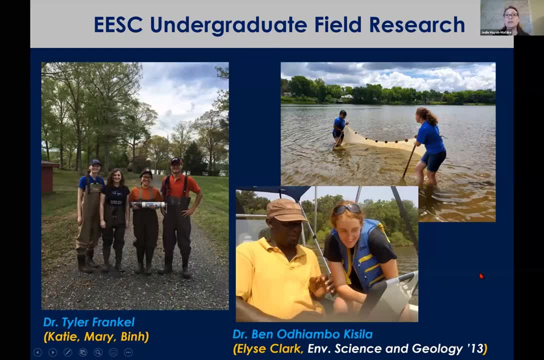 If you live near the study program, how would the housing worker, is that a question for the administration? So the way that that Florida course worked is that students would take the class during a particular spring semester and they would go down to Florida for spring break. So if you could get yourself there on your own, that might be something you could fund yourself. But the basic cost would otherwise be the same. Because you would be going around in vans to various field sites, and you would be taking the class and doing lab work and lecture-based work during the regular spring semester. So it's a regular course. It's just for that particular one, it's a week over spring break that you're down in Florida. 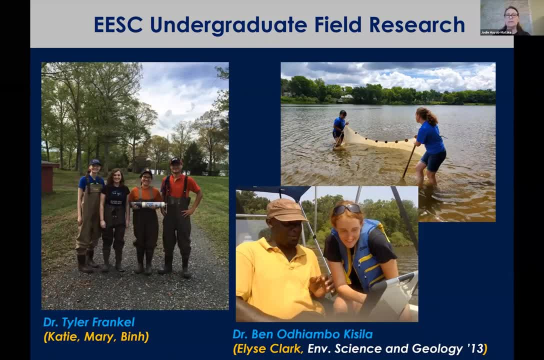 So you would be traveling in the van, staying in hotels, I'm presuming, because it seems like it'd be off, well, maybe camp that time of year. I'm not sure. You'd be traveling with the group, going to the sites that they would be visiting. Yeah. So I don't think it would be possible for you to go stay with your family if they lived in Florida. That probably wouldn't work too well. I hope that answers your question. 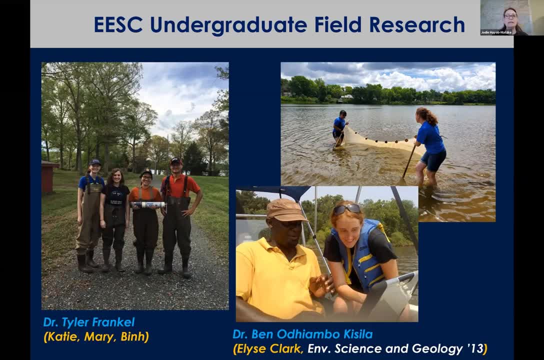 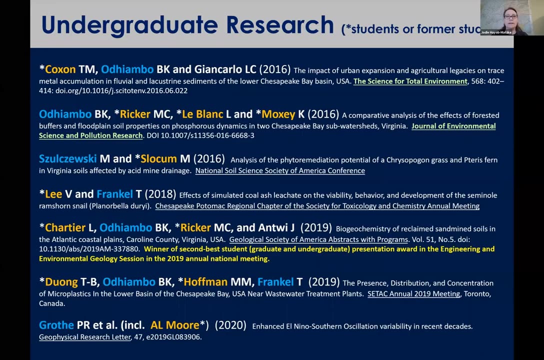 This is a list. This is a very short. I couldn't fit too much on one slide. But what I wanted to highlight is that at a place like Mary Washington, where we're undergraduate only, at least in most of the programs, students are really the main focus. Undergraduate students are the main focus. We don't have teaching assistants. We don't have TAs or RAs teaching the labs. The faculty do it all. We do all the grading. We do all the labs, et cetera. 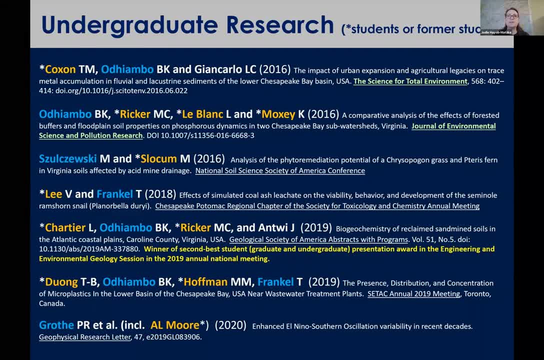 And so the research that we do is is almost exclusively with students. Now, faculty will do some research on their own, but primarily in the Jepson Science Center. 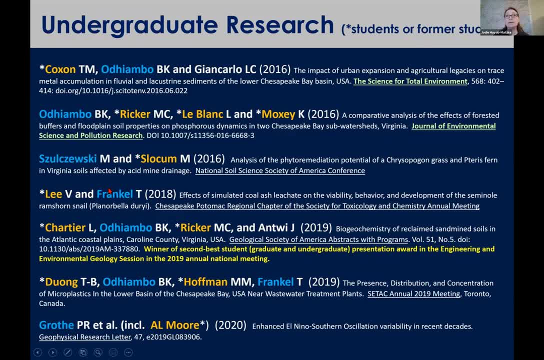 Virtually all of this is done with undergraduate students. So we're seeing in the bright blue are the colleagues from my department. Ben Priscilla. 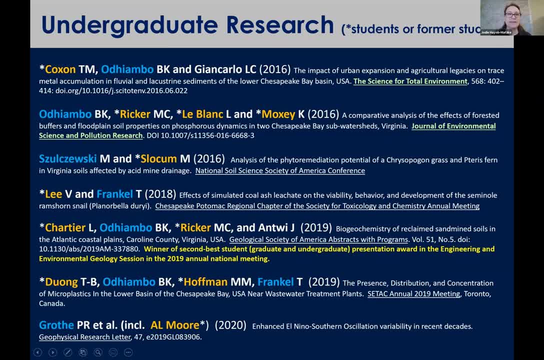 He's Canyon. And I guess the order of the names doesn't matter. So he actually goes by Priscilla now and not Odeombo. That's a little confusing. 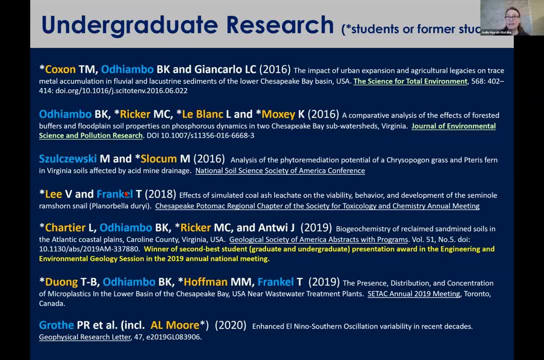 But Ben Priscilla Odeombo is this person. Melanie Szolczewski. Tyler Frankel is our newest hire. He's the ecotoxicologist. He and Ben have co-published and then Pam Groth is our other newest hire. And then the students, the ones that you see in the bright gold are all students. 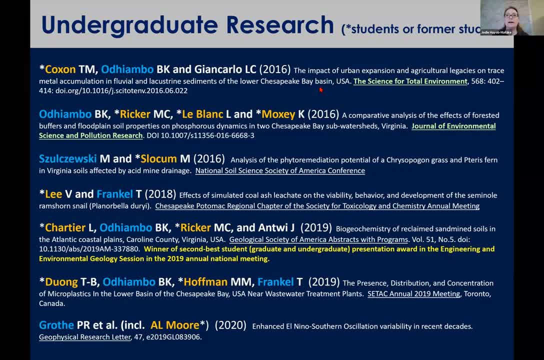 These are all Mary Washington students that have published with the faculty. And so this is a journal article, a journal article. The National Soil Science Society conference. 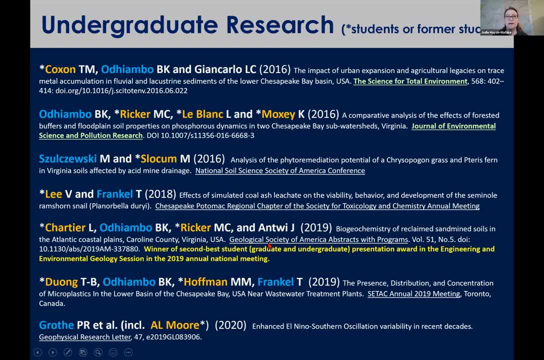 AH & Conlin and 않은 arresting that's been for four months. 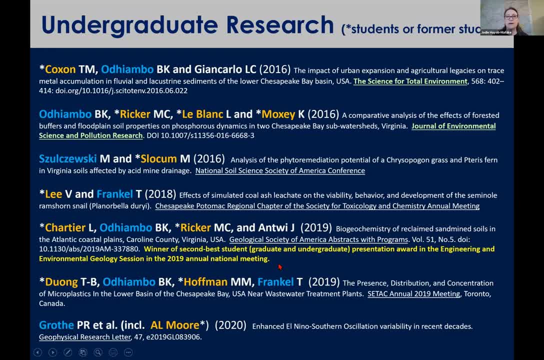 Ben and Lauren and Matt Recker is a former student. He graduated. When did he graduate? Mario curtis. So if you can't hear me, Kelly, let me know. 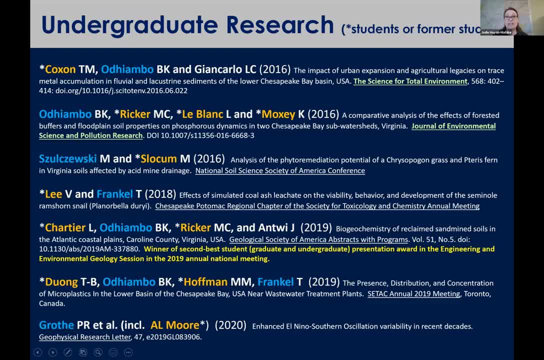 Lauren was the winner of second best student presentation. And she's an undergraduate and she was competing with graduate students and got the second best presentation at this conference. So that was really exciting. 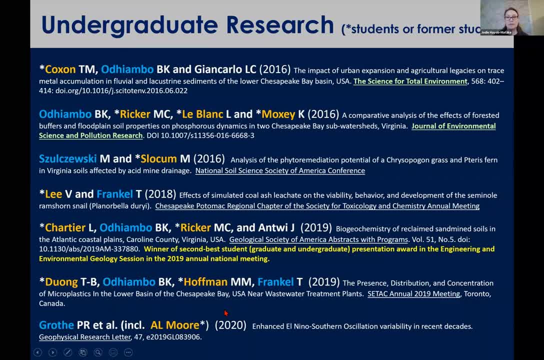 And then Mary and Ben, you saw in the previous image, and I got to move my toolbar so I can read the bottom. 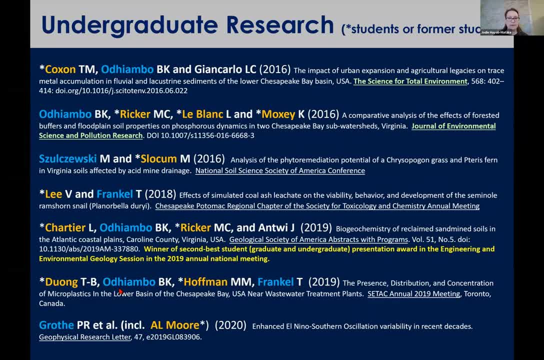 Oh, Andrea Moore is now in graduate school down in Florida. She graduated a couple of years ago. 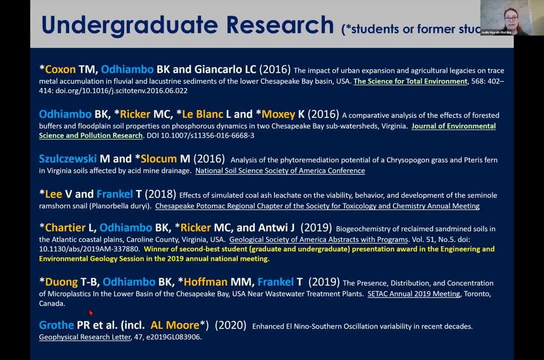 And there were like 20 authors on this paper. So I couldn't list them all. 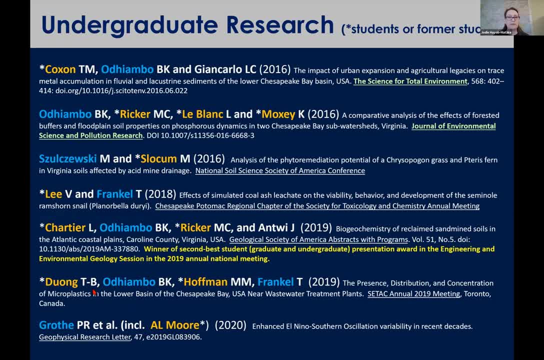 But Andrea was a co-author with Pam on that geophysical research letters publication. So the point here is that faculty publish research articles with students. 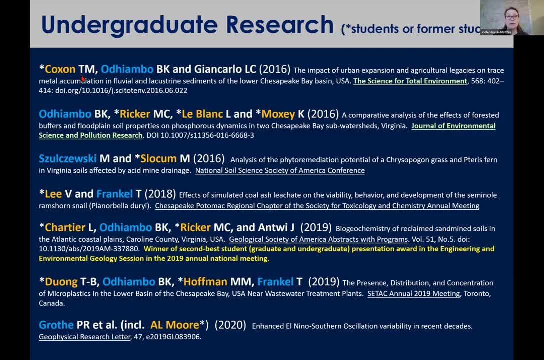 In some cases, Taylor Coxon was really a strong student and really worked hard to get this paper out. 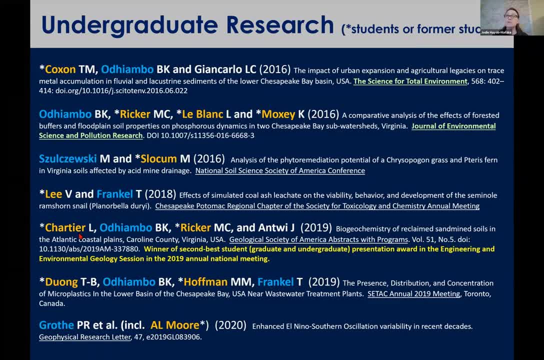 Matt has published papers with Ben where he's been first author. Students are often first. 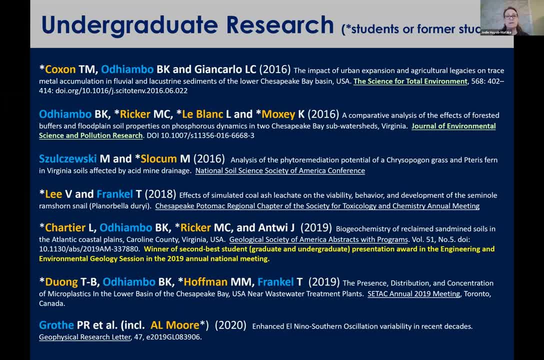 First author is on both research presentations at national conferences, regional conferences, but also journal articles. 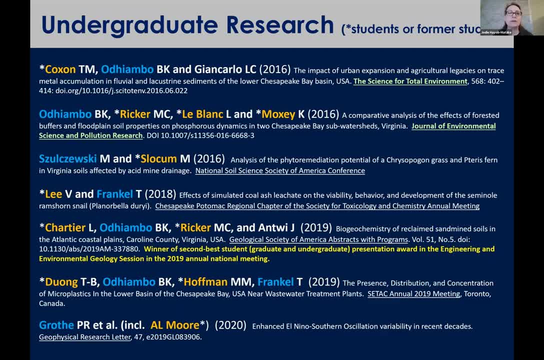 And so it's really up to the student how research active they want to be. There are a lot of great opportunities for students that are really keen to do this, but there's no requirement. 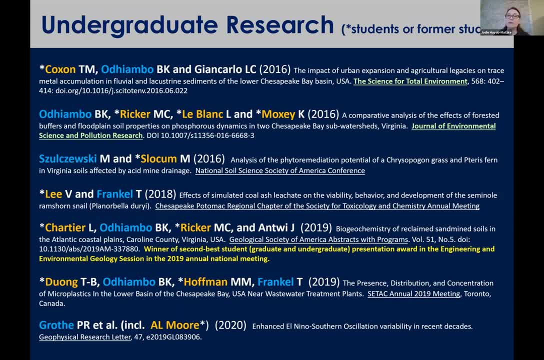 We don't have a research requirement. So if research is not your thing or you don't think you're grad school bound and you want to go directly into the workforce, that's fine too. 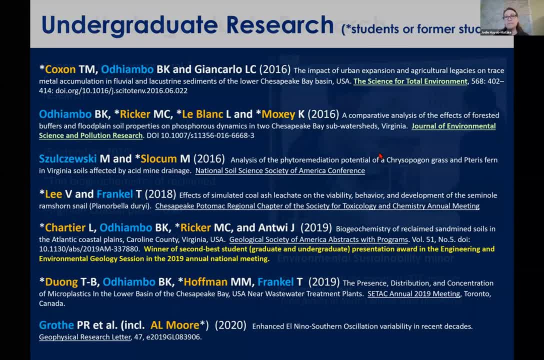 We have a lot of undergraduate research going on. Like I said, this is Lauren Chartier right here explaining her poster. She was a biology graduate last year and she did do our minor. 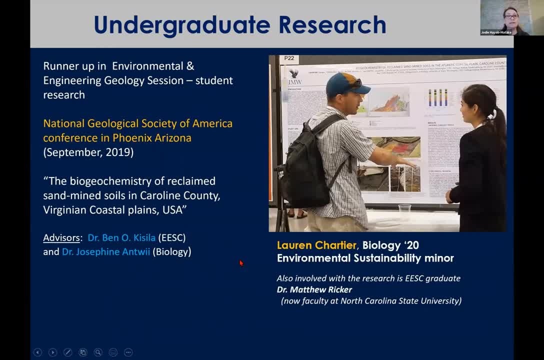 And then Matt Ricker was a graduate from the mid-2000s who's now a faculty member at North Carolina State. And this was Dr. Joe Ontwee from biology. So this was Lauren's presentation. 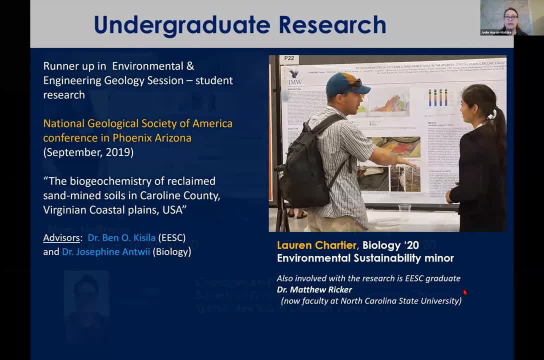 And then this is Mary and Ben presenting their work at toxicology. I can't say that. They've gone to national meetings. This one happens to be a regional one. 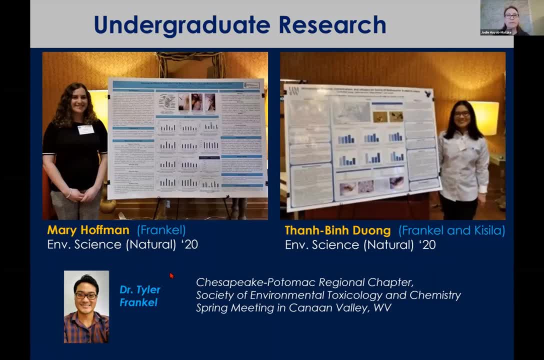 And then this is our latest hire, Dr. Tyler Frankel. 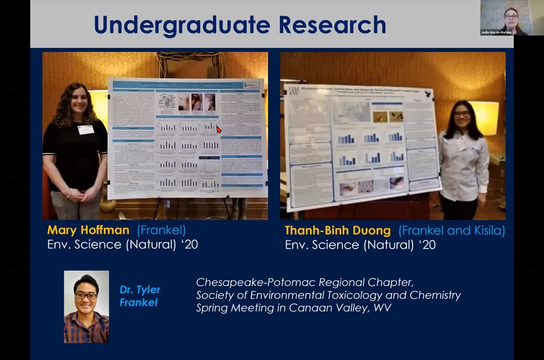 And this just highlights a little bit about our facilities and our funding. Mary Washington in a pre-COVID and a post-COVID year. 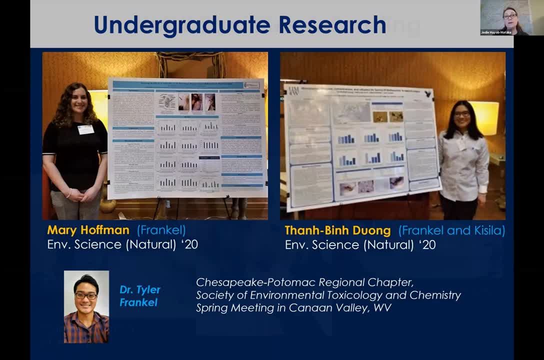 This last year has been a little weird with COVID. We haven't been able to do the things that we would normally do. 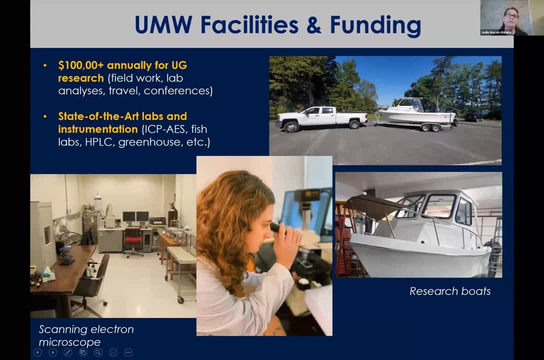 But we commonly have around $150,000. And this is earmarked for undergraduate research. And when I say undergraduate research, I mean undergraduate research. I don't mean just the faculty to do their research. But these are awards that students get. 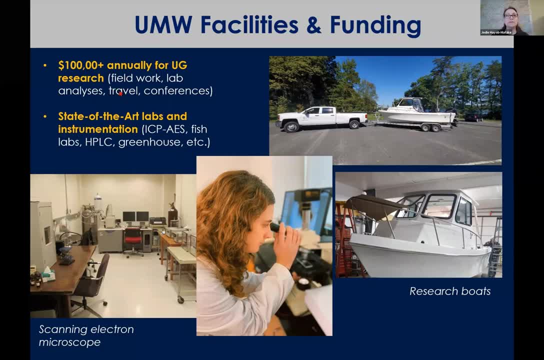 Students write the proposals with the guidance of their supervising faculty member. It can include fieldwork, lab work, travel, conference presentations. 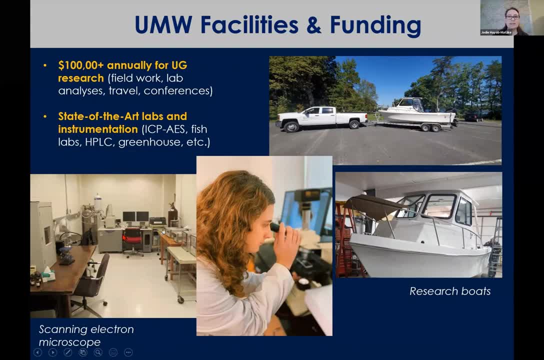 This is our research boat. This is Mary looking down a microscope. We have a scanning electron microscope. We have a lot of great equipment. Really a state-of-the-art kind of stuff that you would find at Virginia Tech or UVA, but you guys get to use it. So if you have questions about what these instruments are, I can certainly tell you. 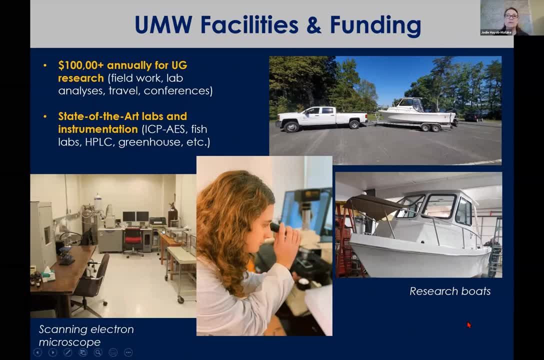 But it's a lot of high-tech instrumentation that students actually get to use if they do research with our faculty. 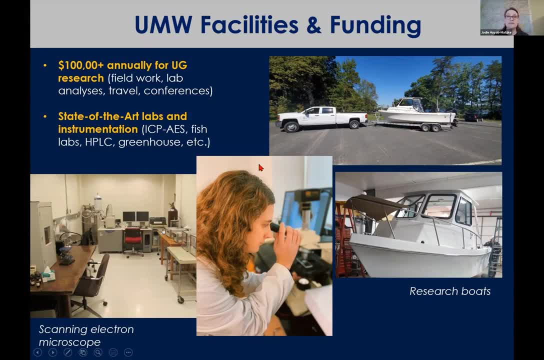 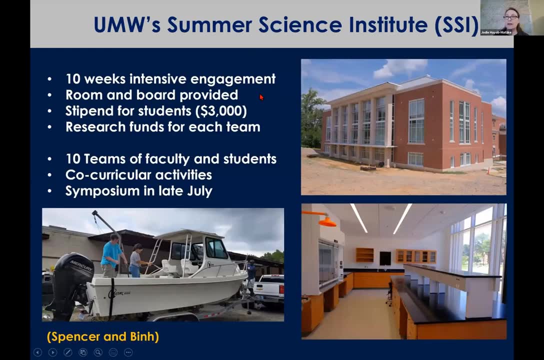 We also have a summer science program, and it consists of teams of students and faculty. So normally we have 10 faculty and 20 students, two students per faculty member. It's a 10-week summer commitment. You are required to. Be on-site. Students get a stipend. They get a salary. 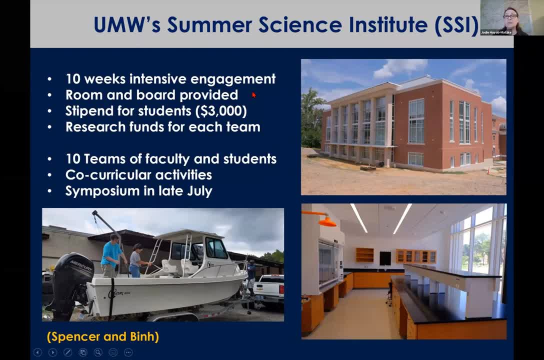 This $3,000 is for the student to use however they wish. Plus they get room and board. 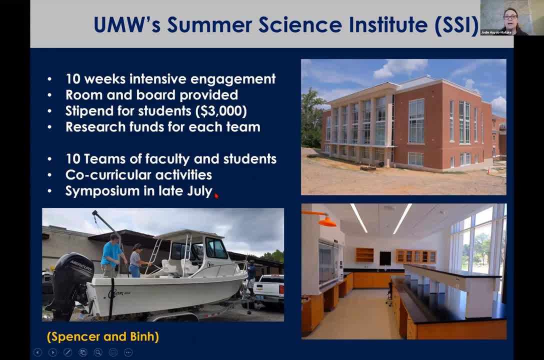 And there's some research money for supplies and fieldwork and so forth. And then there's a symposium in late July where students present their work. 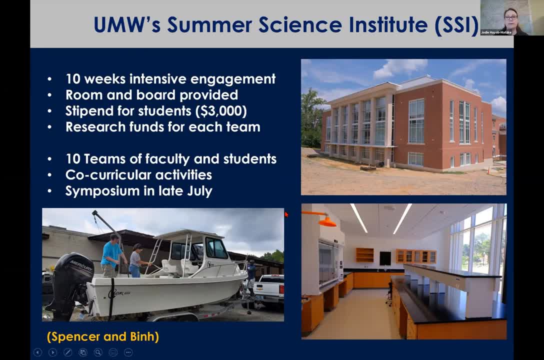 And this is Ben and Spencer on the boat getting ready to go out with Ben to do some sampling. This is the new Jepson Science Center. There's my office right there. 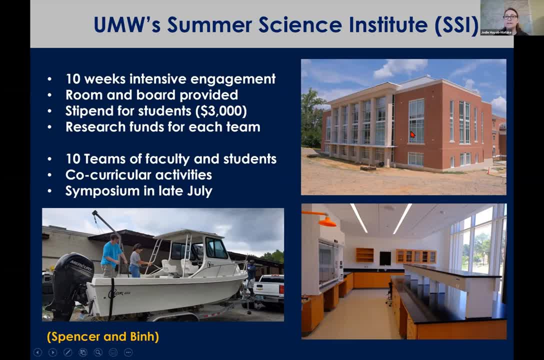 And I'm going to turn it over to Jodi to talk a little bit about some of the things that we're going to be talking about in the next few minutes. 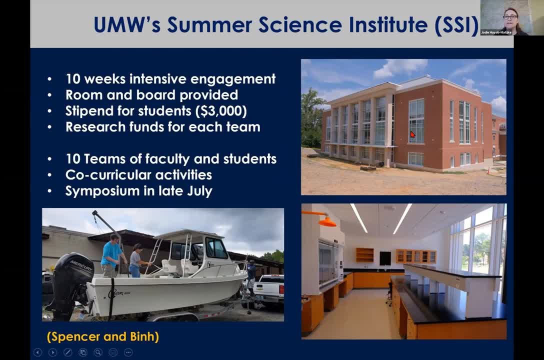 So I'm going to turn it back over to Jodi to talk a little bit about some of the things that we're going to be talking about in the next few minutes. 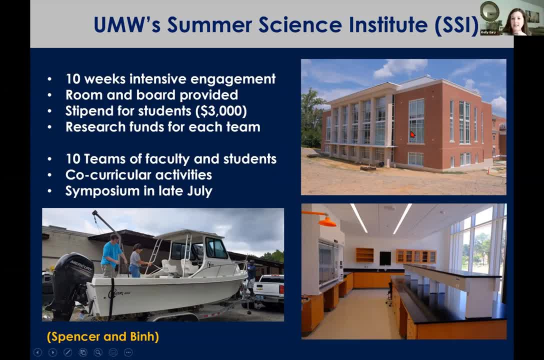 Jodi, you might have frozen again. I can't hear you. Not sure if you can hear us. 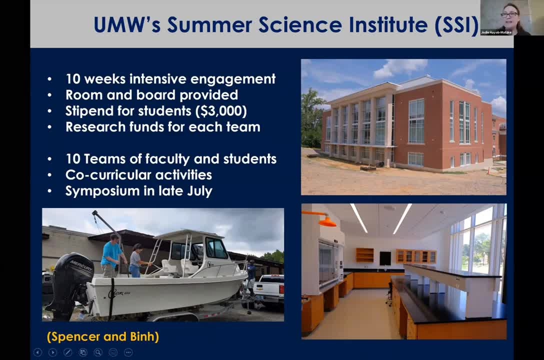 Okay. Can you hear me now? Yes. You're back. Okay. 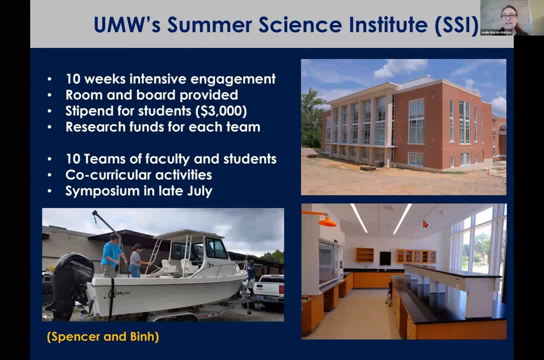 So there was a question in the chat box. Let me go back. Sorry. Sorry about that. That's great. Research is almost all done with undergraduates. Yes, that's true. 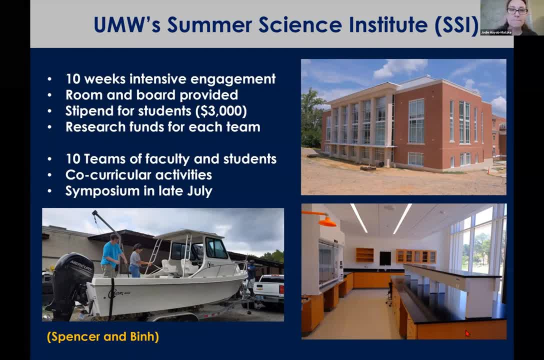 The scanning electron microscope, I was actually one of the PIs on that grant. That was installed in 2005. 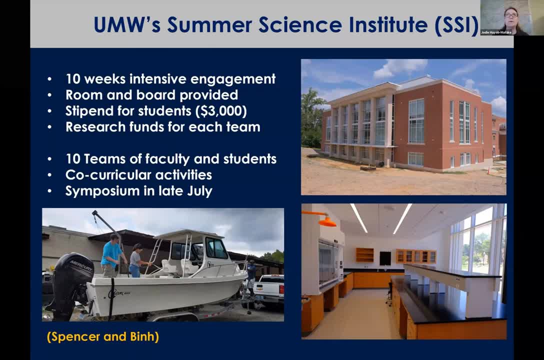 It is a variable pressure scanning electron microscope with an energy dispersive attachment, which means we can get relative or qualitative chemical analyses. The fact that it's an environmental. 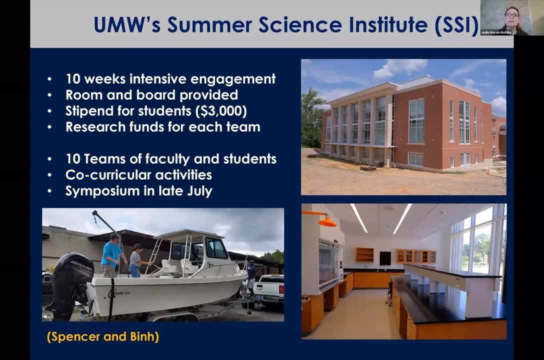 SEM means that you can put sensitive fossils and samples in there without having to do something called carbon coating. So there are different types of SEMs. This one's called an environmental SEM. 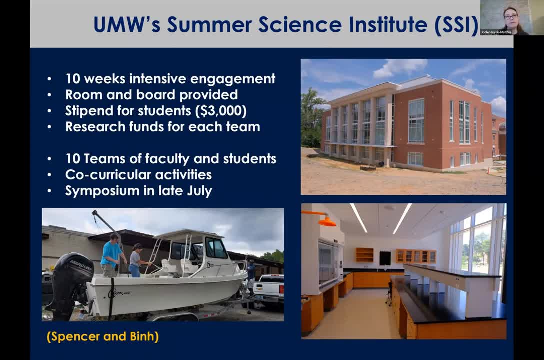 It means it's more flexible. So if you've ever seen pictures of like frogs eyes and flies eyes and flies that are really like hundred thousand magnification, that's the kind of thing you can do with this microscope. So, yeah, Pam growth has used it quite a bit. 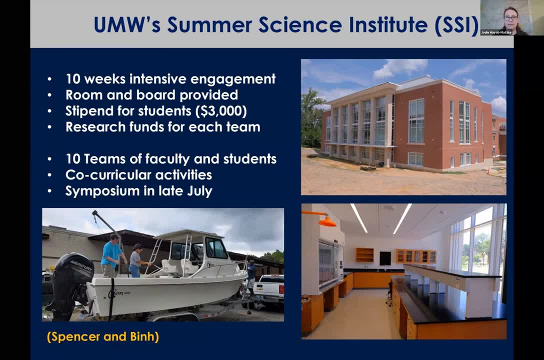 And We're hoping to have a visitor next year. 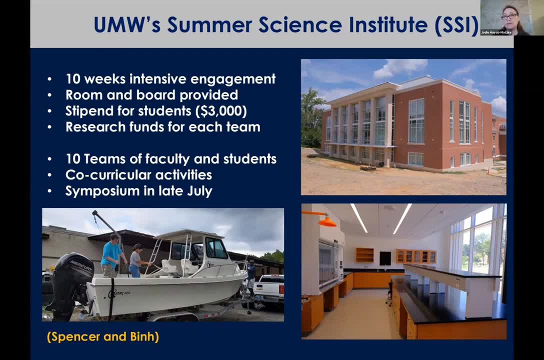 We're still waiting to see if that position gets funded and he's quite interested in using the SEM. So it's used by my department and the biologists quite a bit. Yeah. This is just a vacant lab before we moved in. It's now full of stuff. 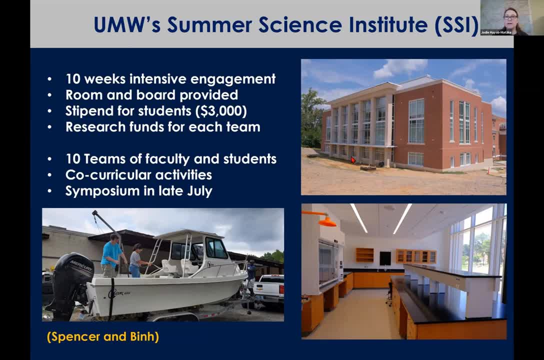 So I was going to say that my department has essentially the entire second and third floors of this edition. Okay. All right. 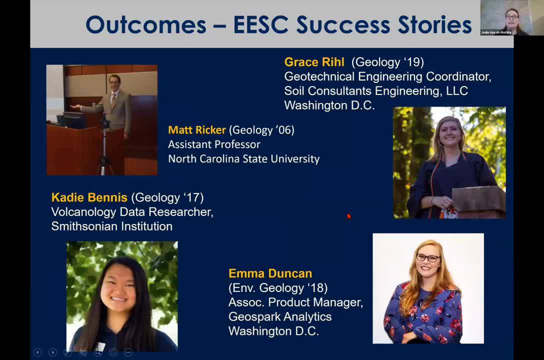 So this is the next few slides just highlight a very small selected set of success stories or students that we wanted to feature. 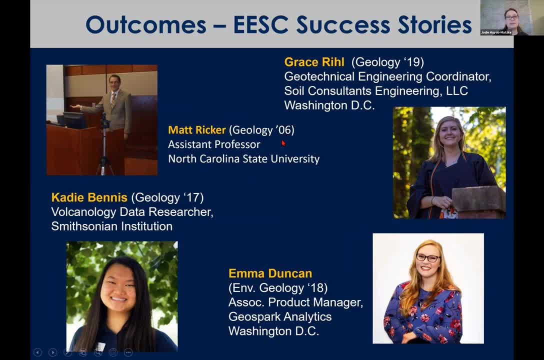 This is Matt Ricker. He graduated in 06. He was a geology graduate and he's now an assistant professor at North Carolina State University. 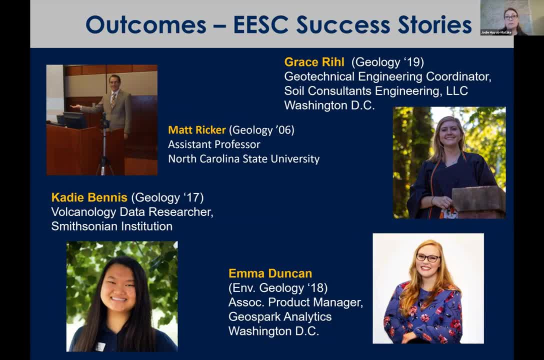 He went up to, I think Rutgers and then Rhode Island to do his master's and Ph.D. 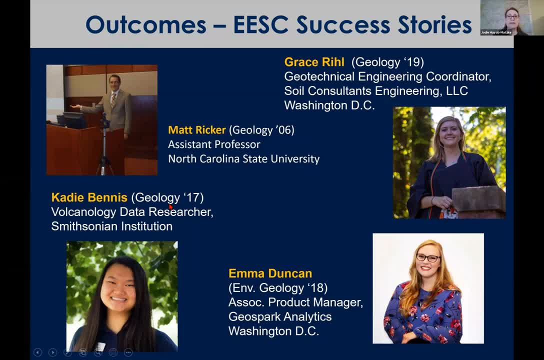 Katie Bennis is was a geology graduate from 2017. So almost four years ago. 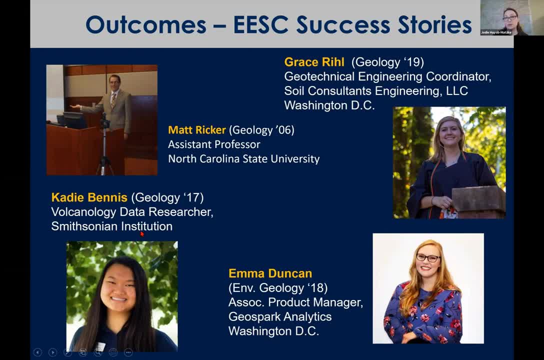 She did her master's. She's in volcanology and is now a data researcher with the Smithsonian. Check the chat. 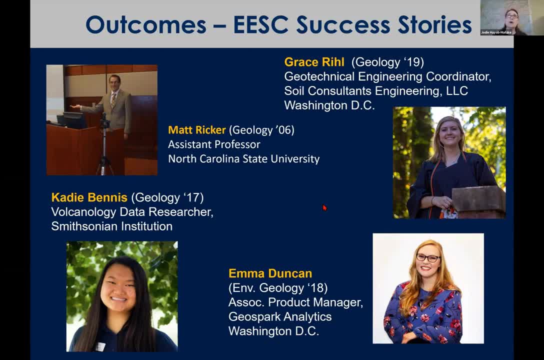 When are kids eligible for the Summer Institute is the question. So we have had sophomores participate. 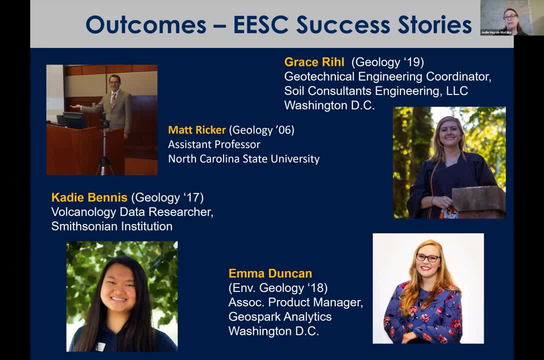 You cannot have graduated. You have to still be continuing the following year. 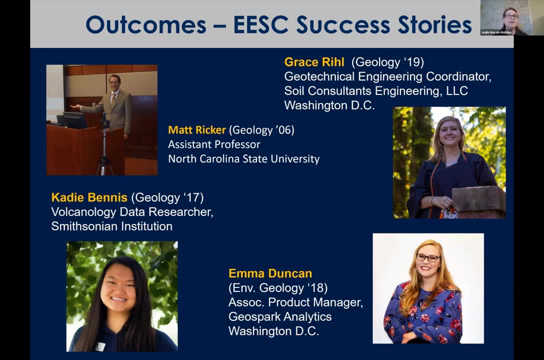 There's no hard and fast requirement that you continue research after the summer program. But the faculty really want you to. That's the whole point. It's meant to be like a seed money. And seed money. 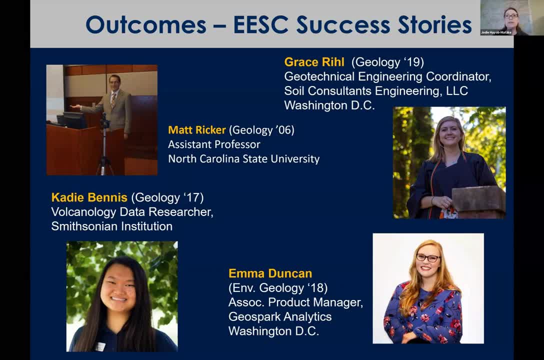 It's meant to be like a seed project to get a longer-term project going. It's really hard in the sciences to get a lot done in 10 weeks. 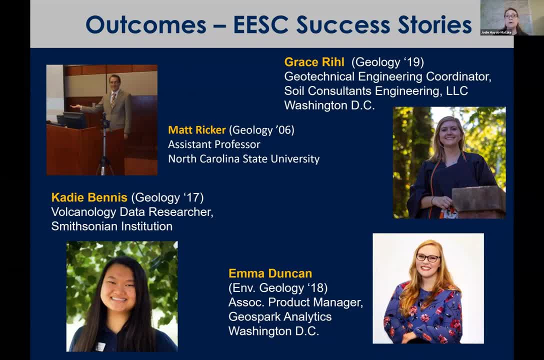 So the ideal candidate for the summer science program would be doing background literature research in the spring leading up to the summer science. You would certainly know by January that you were going to be one of the participants. The teams are selected the previous fall. So you would know by January that you're going to be doing it. 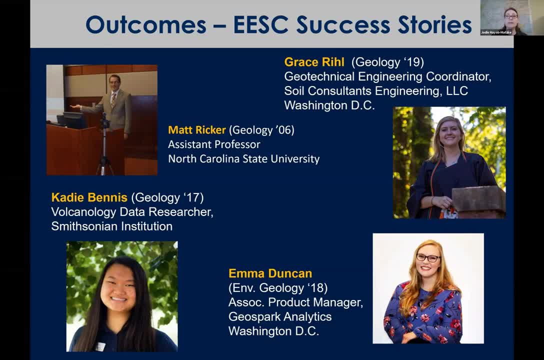 You ideally would be doing background reading and getting ready for fieldwork. You might even be going out and doing some fieldwork. You might even be going out and doing some field sampling in preparation of sending samples off for analyses. 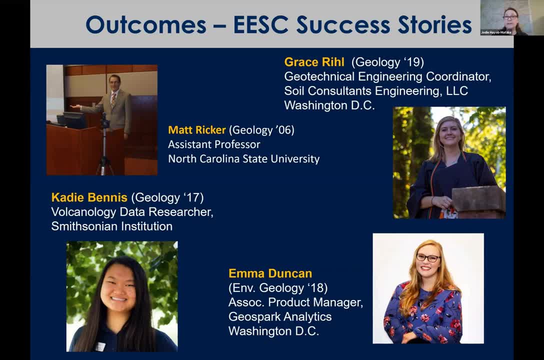 And then in the 10-week summer program, you'd be living on-site or in an apartment. If you wanted to live off campus, you could do that. 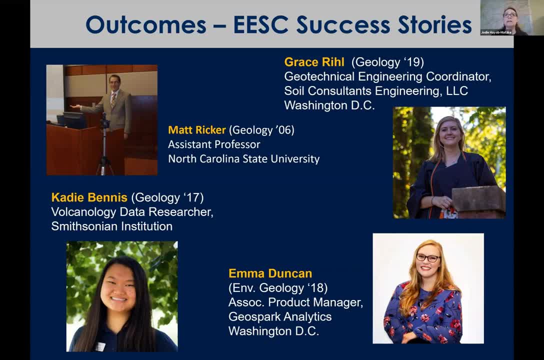 You'd have to pay for that yourself. So some students already have apartments, and they don't want to live on campus. And then they just get the free food. 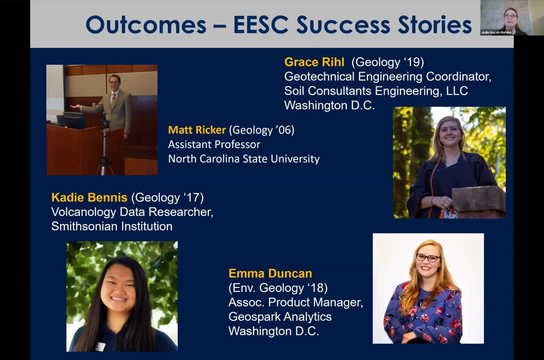 So you'd be doing fieldwork, and you'd be doing lab work and co-curricular activities like hikes and canoeing trips and team building kind of activities. You'd present your research at the end of July, either a talk or a poster session with all of your cohort, the other team members, the other SSI members. 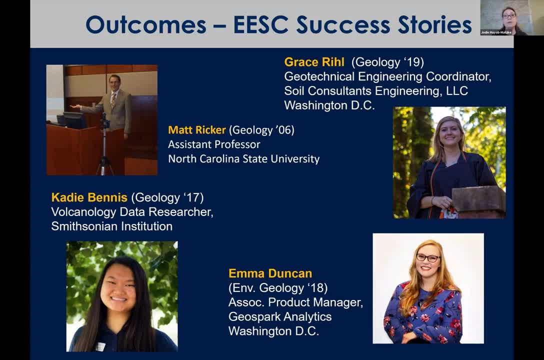 And then ideally, you would continue your research the following year. So most students would do summer science the year, the summer after their junior year. 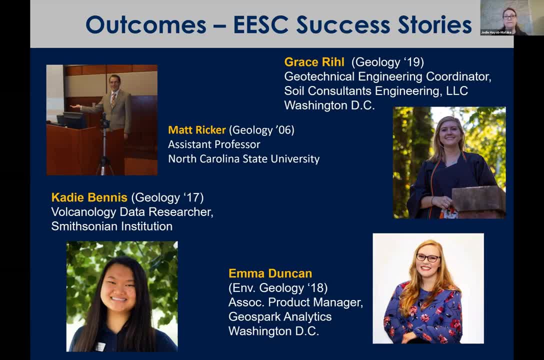 Some do it the summer after their sophomore year. They're really kind of high-achieving, motivated self-starters that are ready for it the summer after their sophomore year. 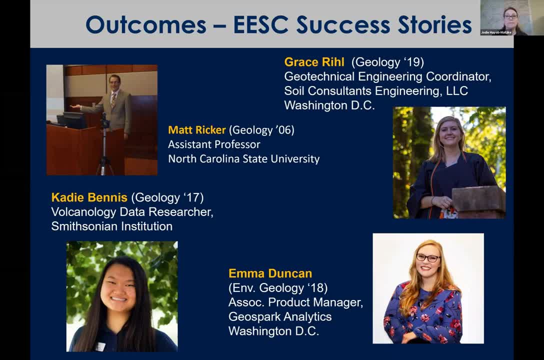 So either after your second year or after your third year. I will say it is a competitive process. 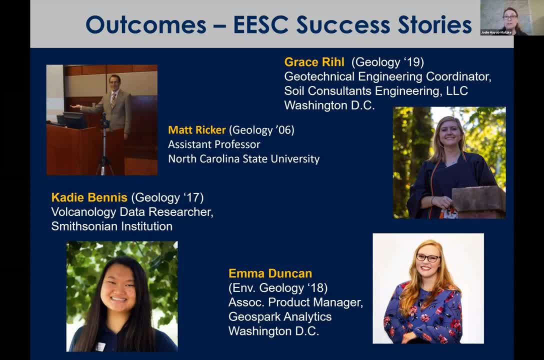 It's not guaranteed. The faculty pick the students. And so if you're, you know, a pretty high-performing, strong student with an interest in research, then, yeah, the chances that you'd be selected would be good. So that's a little different. You know, you're kind of controlling the project. But I'm of an age where, you know, all the projections are different. You know, you're kind of controlling the project. But I'm of an age where, you know, all the projections are different. And the mapping and stuff on the computer did not come easily to me. So, yeah. But a lot of students really love GIS. How much programming is it? It's not a lot. It's one course at the most. And I believe they may have taken that out, which personally I don't think is a good thing. So I would highly recommend that you do it. But I think Jackie Gallagher would know if that's still required. I know they made some changes to the program. But I'm not sure if that's still required. You can also go to the UMW website and just Google GIS, or not Google, just search under GIS certificate in the search box, and you will get lots of information. That will take you pretty much right there. You'll see a link come up that you can click on. You can get a lot of good information, as well as Jackie Gallagher's contact information. Yeah. Kelly just put it in the chat box. It's the CAS is the College of Arts and Sciences, University of Michigan. University of Mary Washington. Yeah. GIS, the certificate, I think. Yeah. Thank you, Kelly. Yeah. So it's right there in the chat. So you can actually click on it and bookmark it right now if you wish, if you don't want to lose that or have to try to write it down. Does anybody have questions about the differences between conservation biology and environmental science? Because I saw that some of you put down conservation biology as potential interests. Yeah. And Kelly put Jackie Gallagher's email in the chat box as well. Yeah. I really wouldn't mind hearing about it. I was actually kind of curious about it. Okay. So I can't say anything bad about biology because that's a great program, too. The two things I would say is if you don't want to take genetics and you want to be more broadly trained, I would do environmental science. So a lot of the coursework, if you like literally compared course for course, the conservation biology major was kind of modeled after our environmental science major, the natural track one that we have. The difference is that because theirs is more of a biology major, you do have to take genetics. And in our major, you don't have to take genetics. But you do have to take hydrology, which is the study of surface and groundwater. And given that a main focus of environmental science is environmental science, you do have to take genetics. of environmental consulting, which is where a lot of the jobs are, is the transport of contaminants. And given that contaminants are transported usually by either wind or water, I think hydrology is just critical training for anybody that plans to work in the environmental sector. So I would argue that our major is a broader training, a better training, more flexible for getting a job. But I can't argue with anyone who wants to work with wildlife, for example. I mean, conservation biology is really popular. It's just more hard to find a job. So yeah. And you could do both. You could do a conservation biology major and an environmental science major. It would not be impossible, but it would take careful planning because you can only overlap nine credits between two majors. So if you're going to double major and that's... I was just about to ask that is if you take both majors at a time, are there many overlapping classes that you can take? And remember you mentioned like you don't, you have to do a hydraulic, and for yours, but are there any similar overlapping classes you can take for both majors? There are, in fact. So as a biology major, you have to take the full year of introductory biology, but it doesn't count in the major. And likewise, for our environmental science majors, you have to take the full year of introductory biology as an embedded prereq. And then if you're a natural track, if you go to science, the natural track, natural science track of the environmental science, you have to take effectively four semesters of biology. You take the year of introductory biology, you take their two, their three credit biology 210, which is introduction to ecology. And then you have to take what's called an upper level ecology. And there are about five choices. The ecotoxicology that my colleague teaches is a choice. So you don't have to take biology for the fourth requirement, but you could do animal ecology, plant ecology, biology of fishes or ornithology. Those are the other courses that count. So you could do our toxicology. If you wanted to double major in both conservation biology and environmental science, natural track, it would be a little tricky because I think a lot of the courses would overlap. And then you would just have to, we'd have to sit down and map it out. There'd be, if it's a required course for both, then sometimes it's not possible to double major because there would be automatically two majors. So if you wanted to double major in both, then you would have to sit down and map it out. There's a whole lot of things that you can do that don't overlap. And I don't know yet. We haven't had any students do that because their conservation biology majors pretty new. It's only about two, a year or two years old. So no one's attempted to do conservation biology and environmental science, natural track. So I don't want to promise that it's possible. I think we'd have to sit down and literally look at all the overlaps. It just means you have to take enough electives and enough other stuff to get the double major. And that's a university requirement. That's not specific to my department and all Universities have these restrictions, by the way. It's not unique to Mary Washington. No university is going to let you get a double major just by taking a few extra classes. That just doesn't happen. There's no physics. The environmental science is three semesters of chemistry. It's the year of introductory chemistry plus a third semester. And we have an option in my program called environmental geochemistry, which most of our students prefer to take. And then if you do the social track, it's three semesters of biology. You stop with that three-credit Bio 210. Or if it's the natural track, you take a fourth semester of biology. So it's either three or four semesters of biology. Both tracks have three semesters of chemistry. There is no calculus requirement, and there is no physics requirement for anything. Nothing in my department requires calculus or physics. We recommend. If you're interested in grad school, but we don't require it. I have to go out is really because I have an appointment, but I really did enjoy it. Thank you. Thank you. Have a good evening. Let's see. Gabriel was asking one more question here. What is if you, if you need to log off and go, please do. It is seven o'clock, but I was going to answer Gabriel's question. When would you say students considering both options have to choose between them? Not for a while. Between, I don't know if you mean between conservation, biology and environmental science, or if you mean between our two environmental science tracks, but certainly between our two environmental science tracks, the coursework that you would take in the first year or two is the same. So certainly for the first year, it wouldn't matter. The recommendations of the coursework would be the same, regardless of which track. Yeah. Between environmental science, natural track and conservation biology, it would be even more similar. So. It would be the year of intro bio. Well, I guess the difference is that if you wanted to do our major, we would recommend a year of introductory and you'd need to do EESC one 10 and one 20, your first year, ideally. And if you're going to go conservation biology, you'd be doing biology and probably chemistry. Whereas if you were going to do our program, we would recommend our two courses in the year of biology and hold off on the chemistry. So in terms of getting the EESC one 10 and one 20. Yeah, in that regard. Yeah, you're the more I think about it, you probably would, but you could take the one 10 and the one 20 and still switch over to conservation biology. And those credits aren't lost. They count towards the one 20 to graduate. All students take roughly a third of their classes or credits are in the major. Roughly a third are gen ed and roughly a third are pure elective. The one 10 and one 20 is the year of introductory environmental science that my department offers. So even if you took my one 10 and one 20 and then decided you're going to be a conservation biology major, probably some of the electives that you'd want to take for the conservation biology major would either require those two courses from my department if you wanted to take an elective in my program, or it'd be really helpful. But even if you didn't need the one 10 and the one 20, which is seven credits together, you would find that those credits count towards 120 that you need to graduate. They would just be counting as electives. So they're not wasted credits, they count for something. Everything counts for something. Nothing is wasted, it goes towards the one 20 to graduate. If that makes sense. 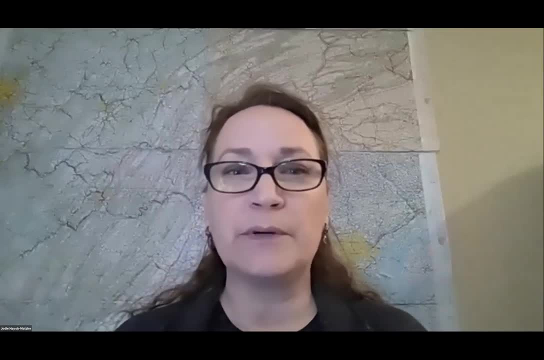 I hope I answered your questions, Gabriel. You can always email me as follow ups if you still have questions. It's a pleasure to chat at you all. 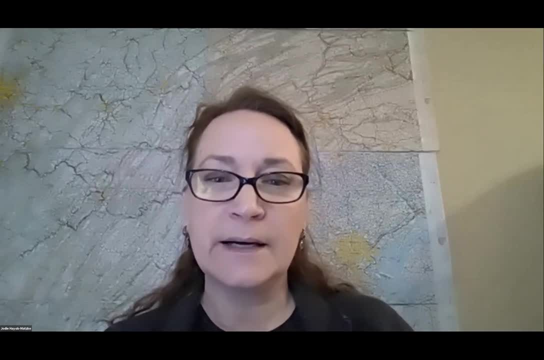 All right, have a good evening, everybody. We'll see you in the next email if you find that you do have questions. Thank you. You're welcome.